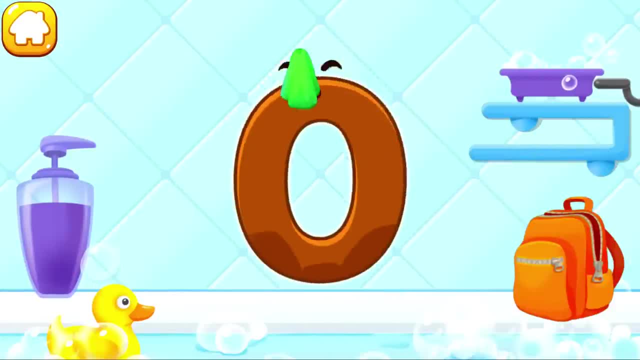 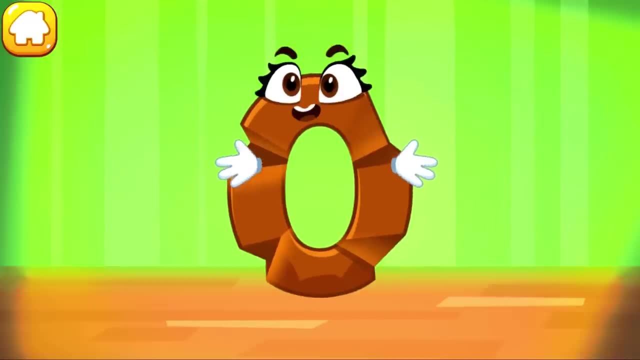 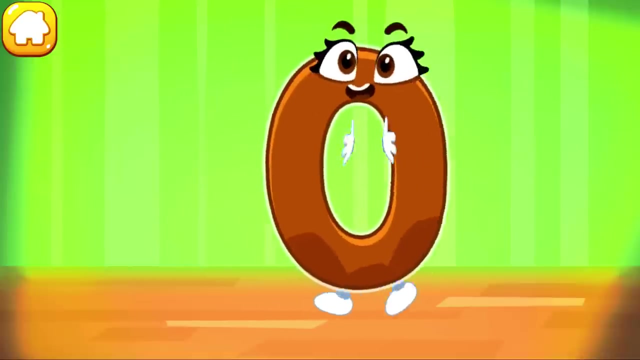 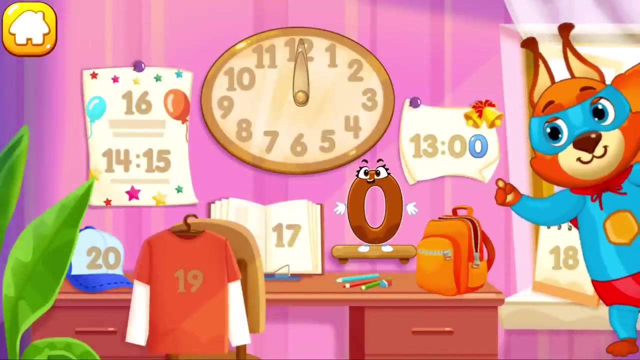 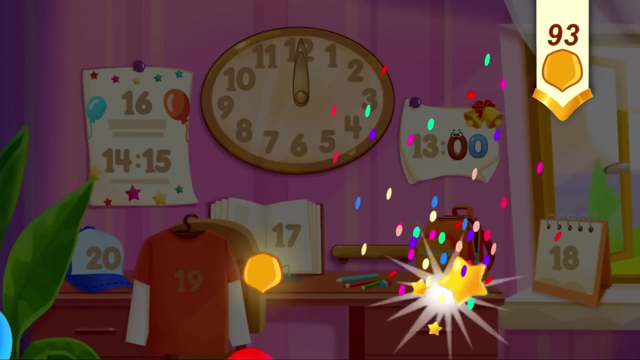 Wipe the figure with a towel. Done, I earned the number zero. Beautiful, Put the number zero in its place. Now I'm safe. You've earned a nut for the squirrel. The wind blew away the number one, The number one, straight into the sea. 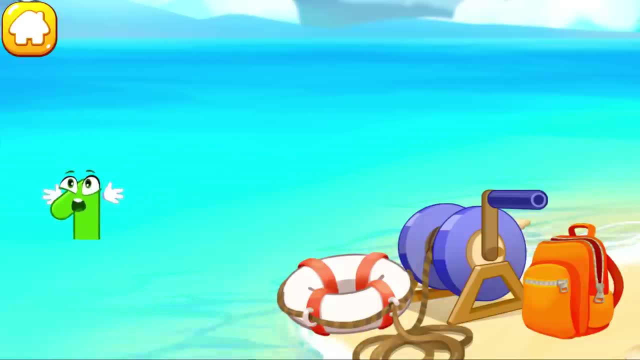 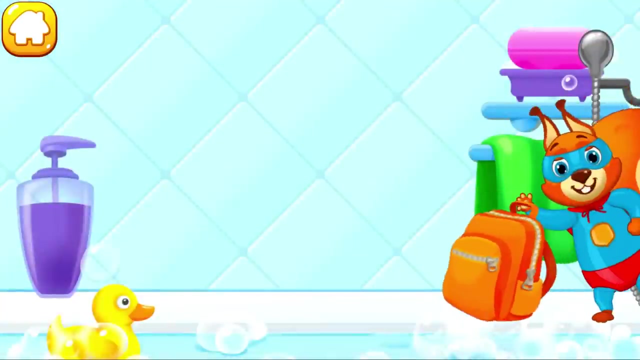 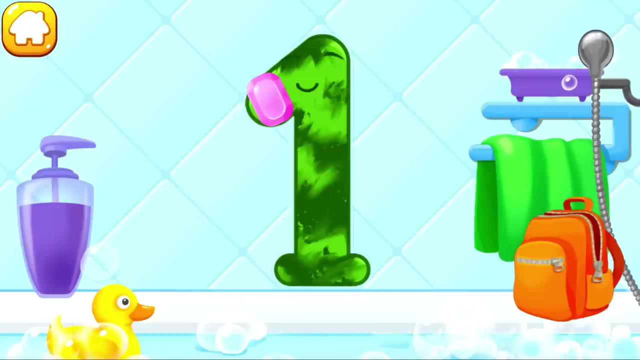 Help it get out. Throw a lifeline Caught it. Press the blue spool to pull the number one to the coast. Cool Wash the number one. First apply soap on a number. Then apply soap on a number. Next spread out the rope to block them. 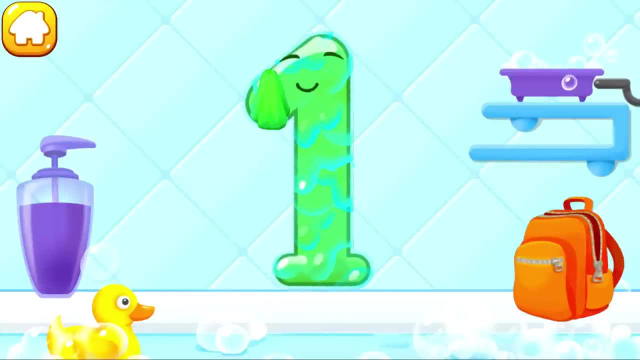 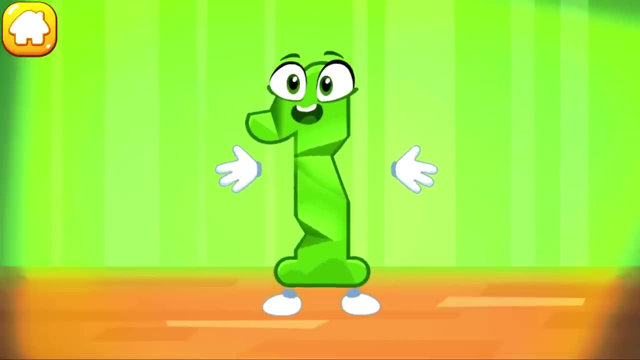 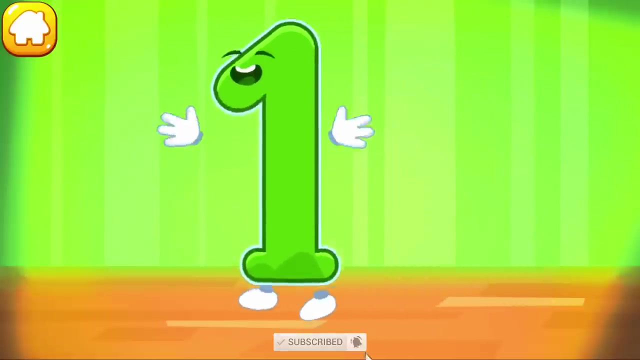 Use your hands to help the number one to get away from the water. Take out the rope And wrap and tie the rice, Violet and goals, Addكa, thfav and cover the number one on three hands. Keep it tight. Questions: Try a few and let me know what the answers are in the comment section. 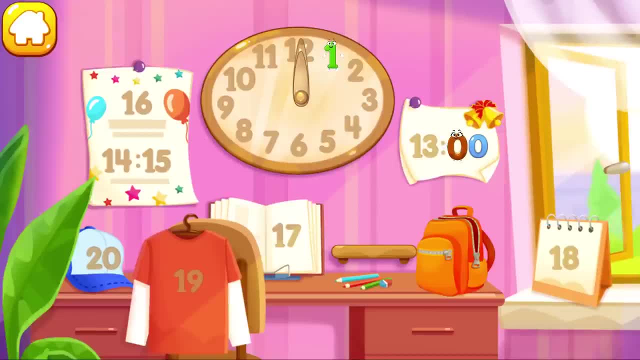 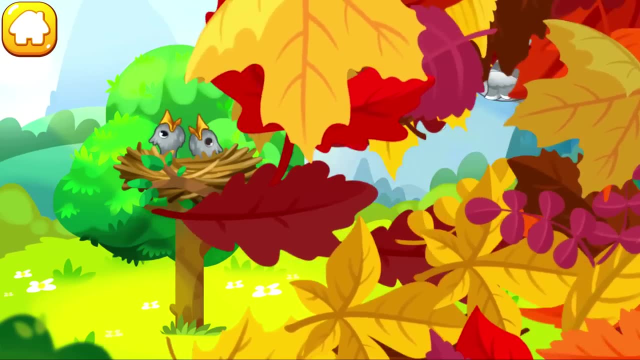 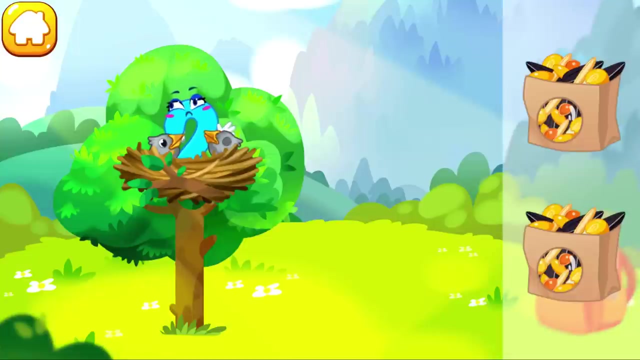 Awesome. I know you want to know what the numbers will be, but now think about it any time to learn the rules. I've learned the number one: squirrel. the number two was caught by a bird and carried to its nest. let's feed the hungry baby birds with some seeds. 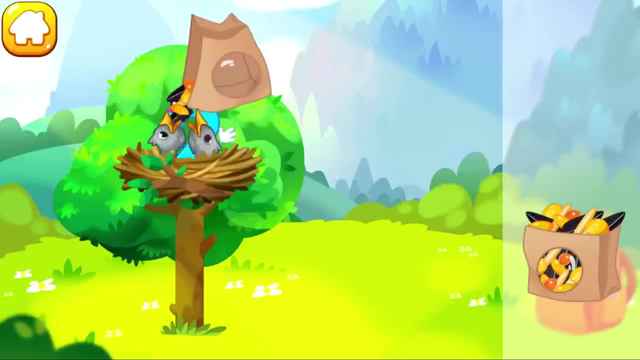 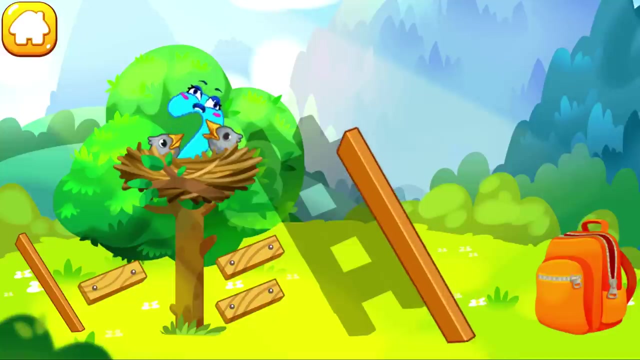 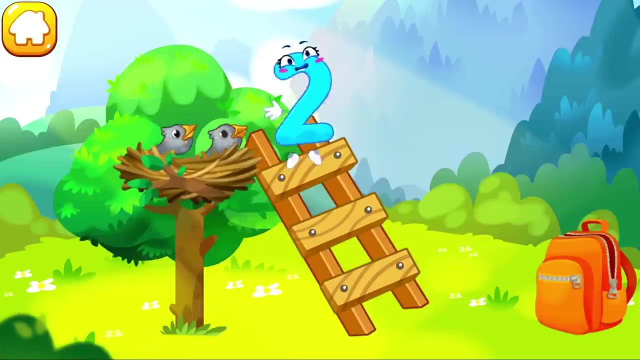 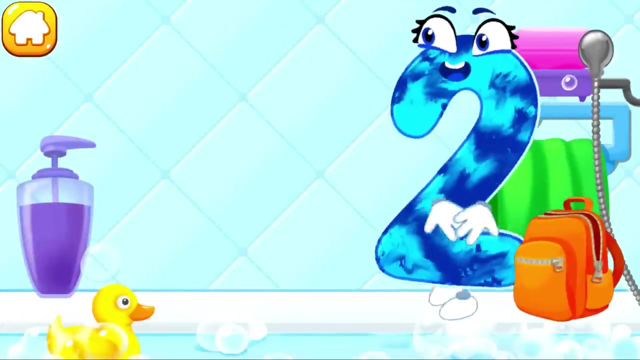 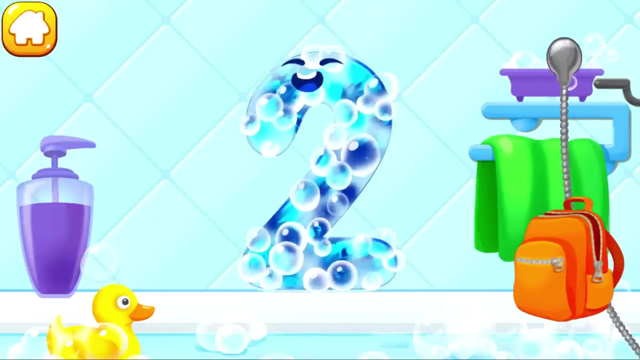 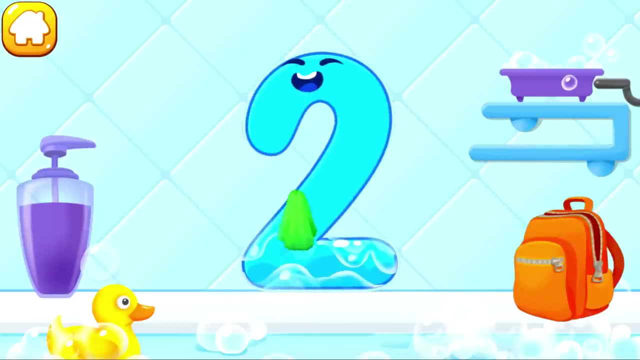 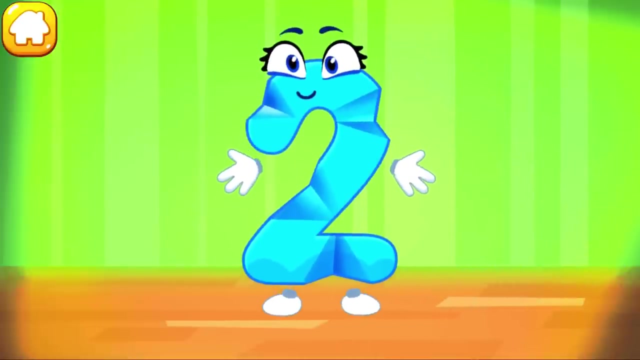 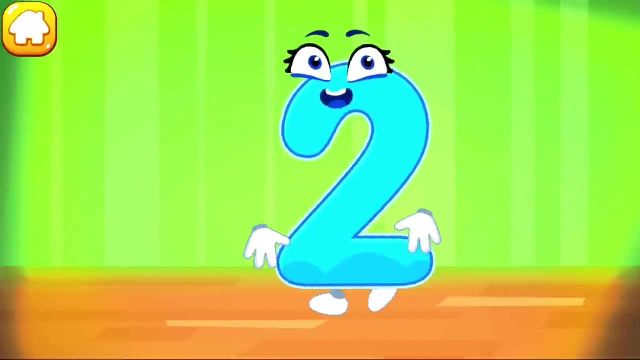 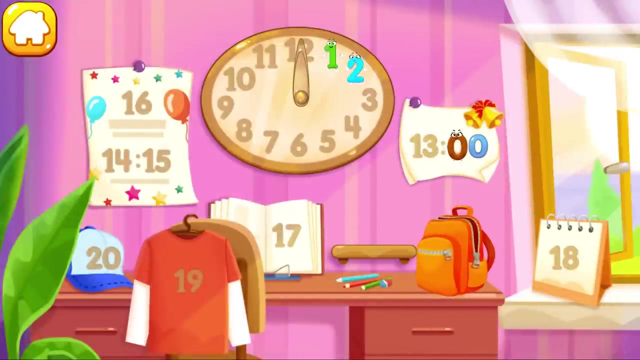 now assemble the ladder so number two can come down. assemble the ladder from the part. good job. wash the number two with soap first. wash away the soap with water. wipe the figure with a towel. good, iron the number two ready. put the number two in its place. thanks for the help. take a nut for the squirrel. 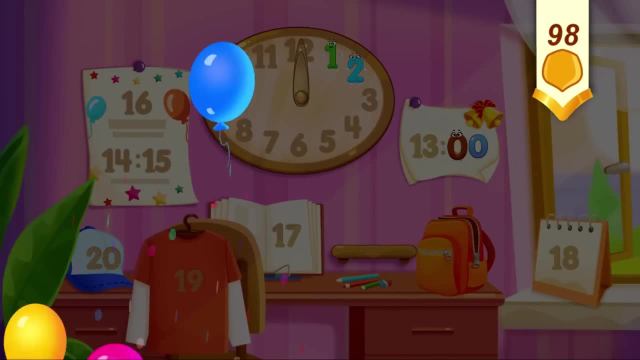 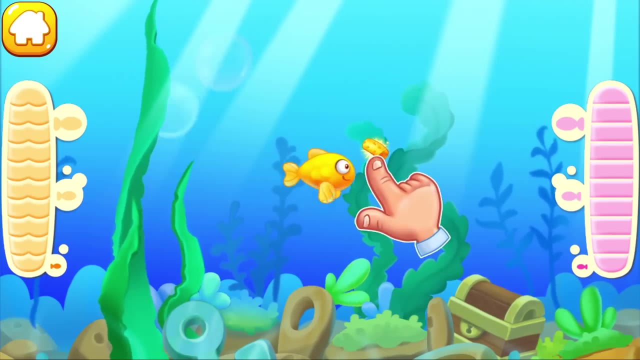 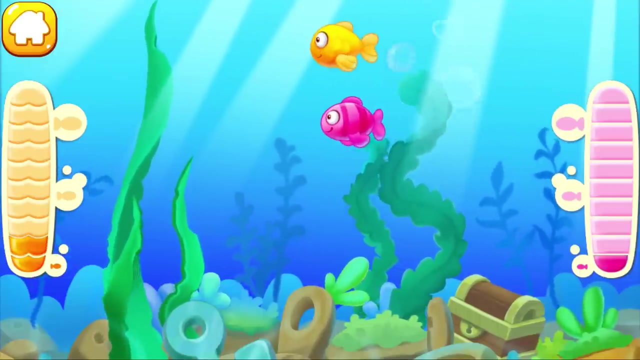 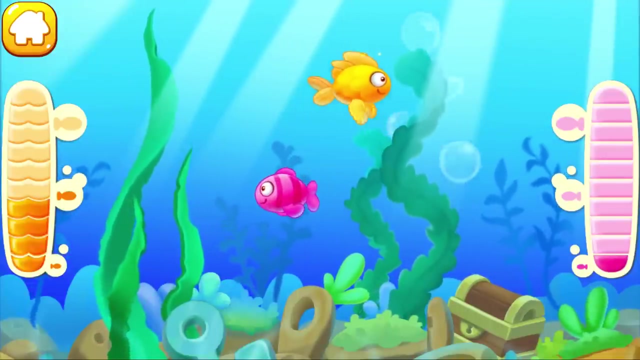 let's help our squirrel feed the fish. tap on the food for the fish to eat it quicker. the fish hasn't had enough yet. tap on the food. wow, the fish got full and grew up. Wow, the fish got and grew up. the fish got full and grew. you can see how it grew J. 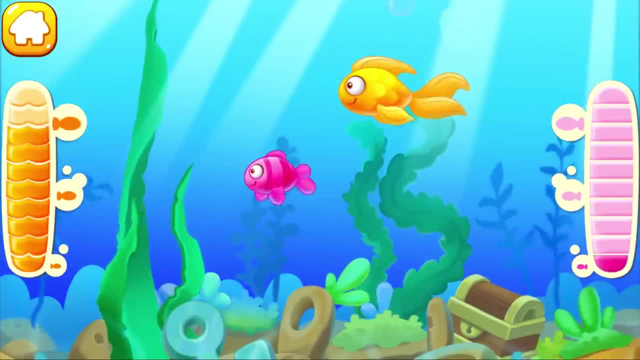 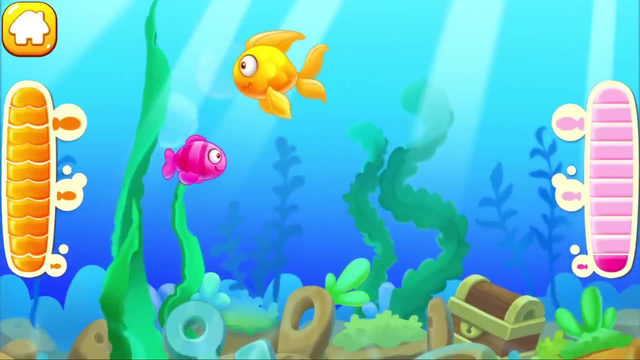 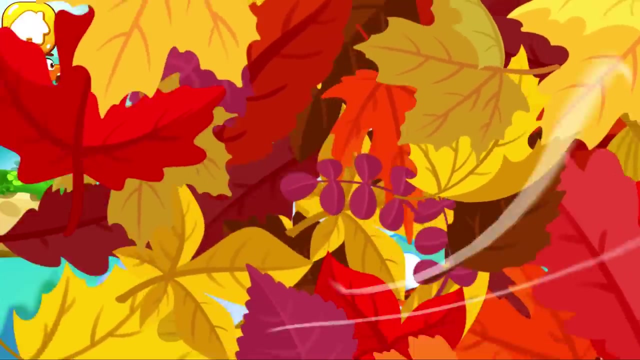 waaauw, this little fish has swimming hood. the bird is very happy now while the alignment水- i see the fish catch eels. that's faster overlooked. do you try fishing? number three got to the other side of the abyss. make a cloud road so the number can. 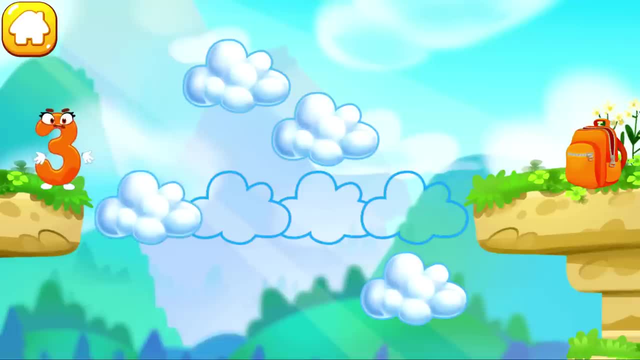 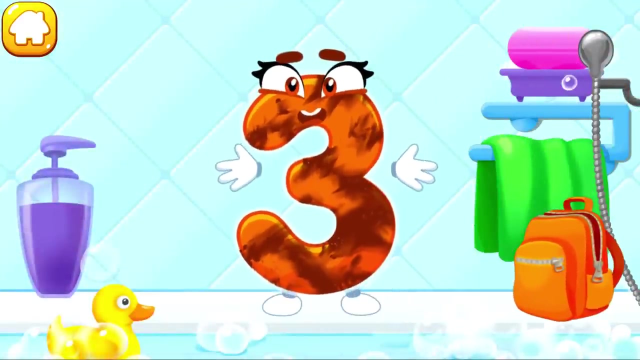 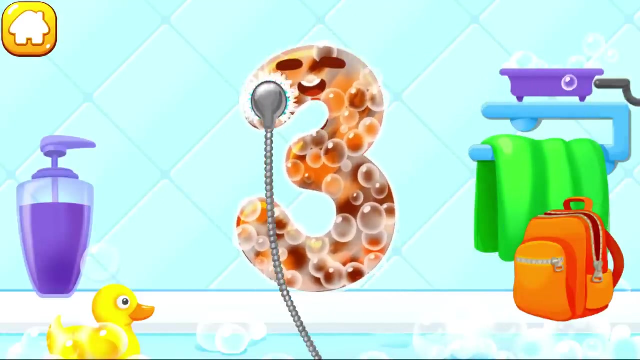 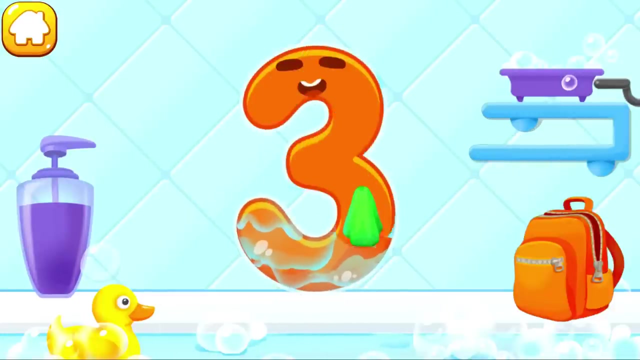 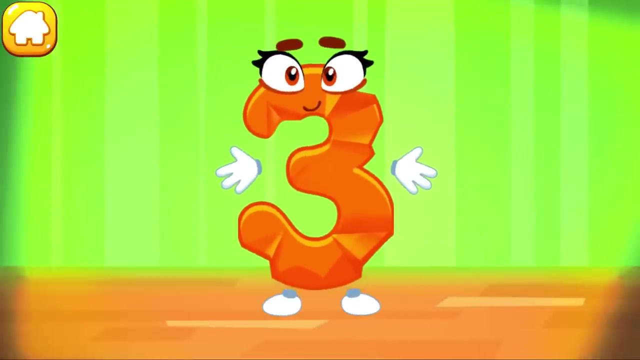 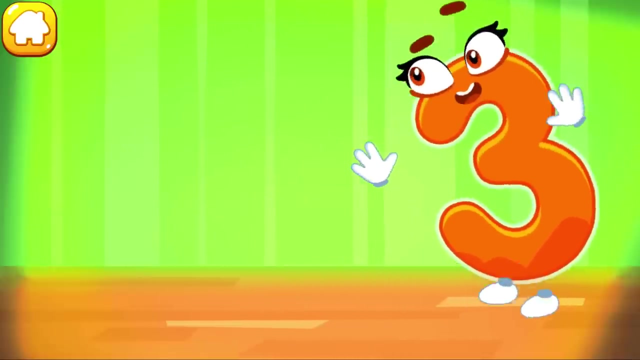 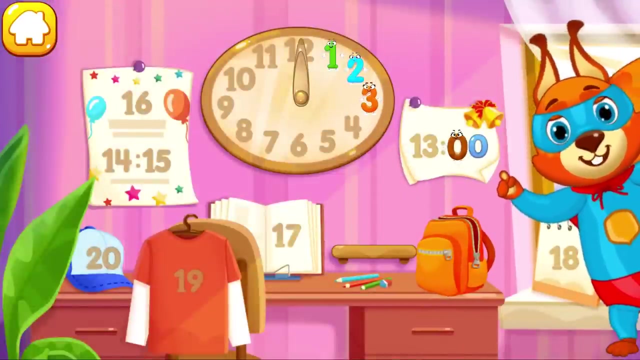 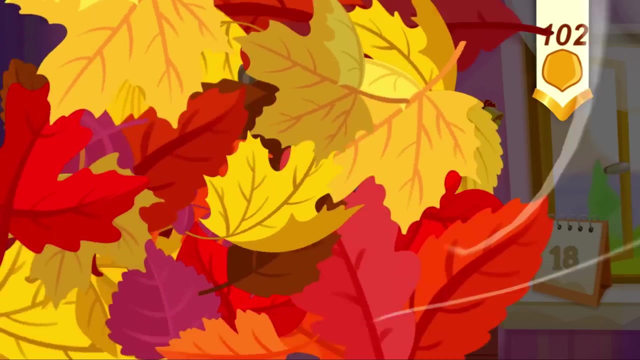 come to the backpack ready. wash the number three with soap first. wash away the soap with water. wipe the figure with a towel. beautiful iron the number three done. put the number three in its place. thanks, you've earned a nut for the squirrel. the vegetables in the squirrels garden need a lot of water to grow. well, let's. 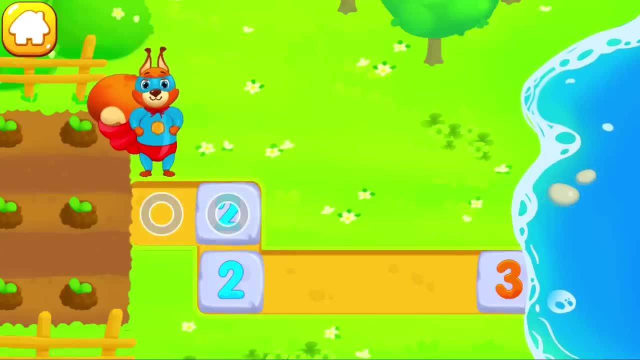 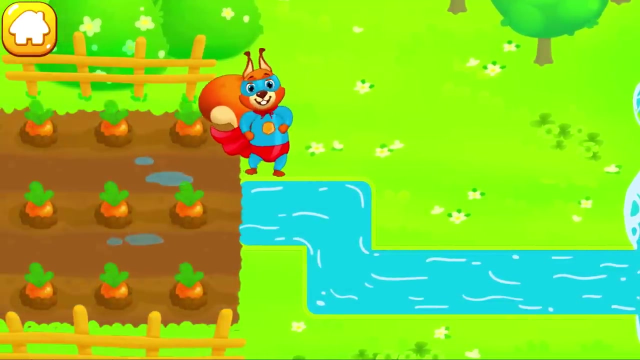 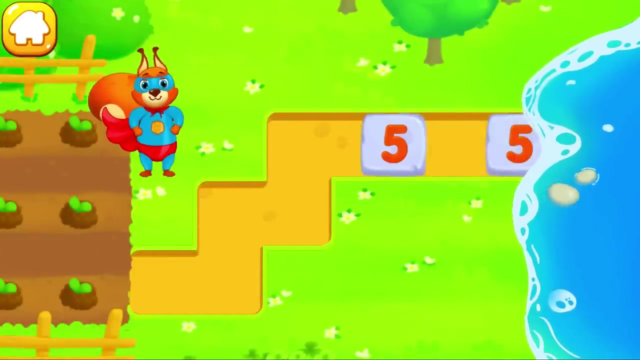 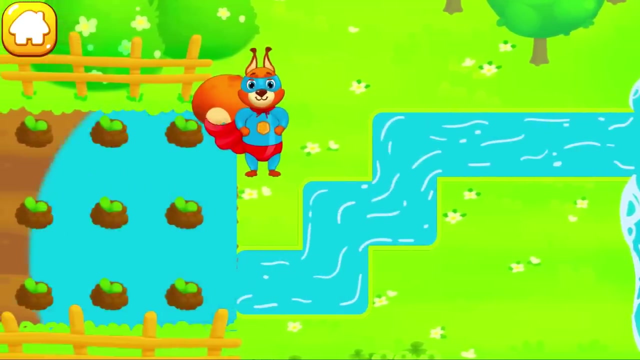 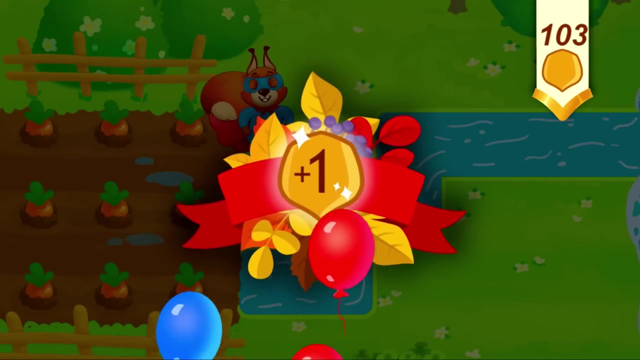 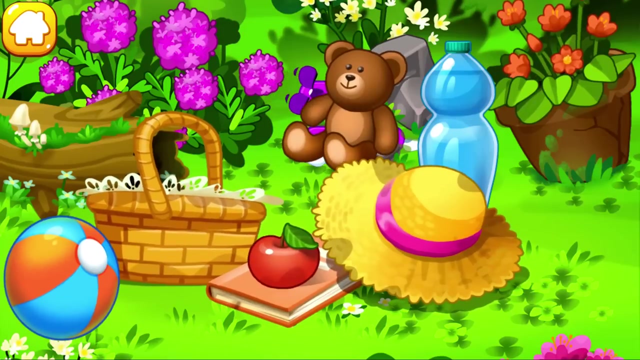 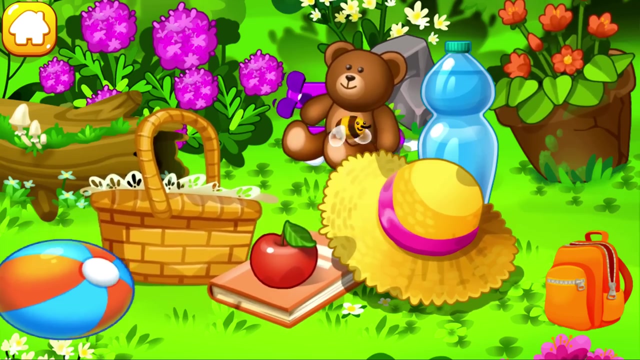 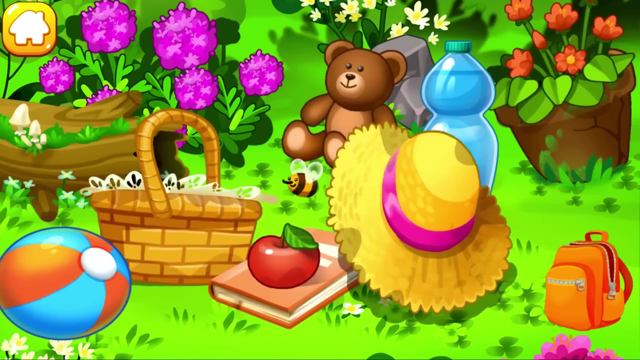 bring water to the garden. swipe the screen to join the same stones. beautiful you, you're doing great. take a nut for the squirrel. the number four hit the clearing tired and fell asleep. where's number four now you? number four is playing hide-and-seek, find it. 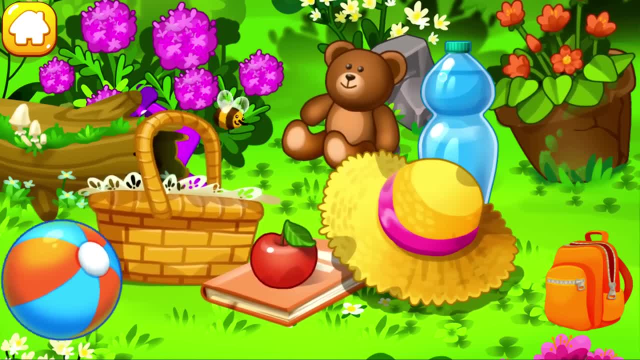 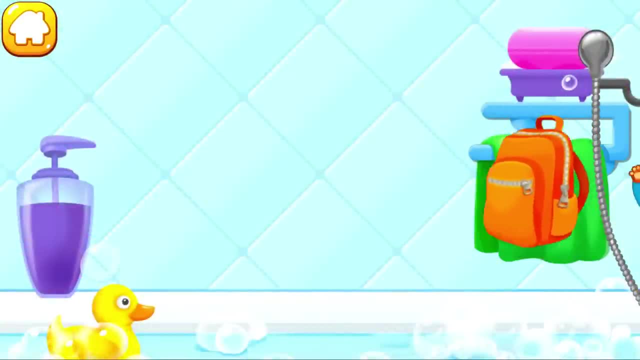 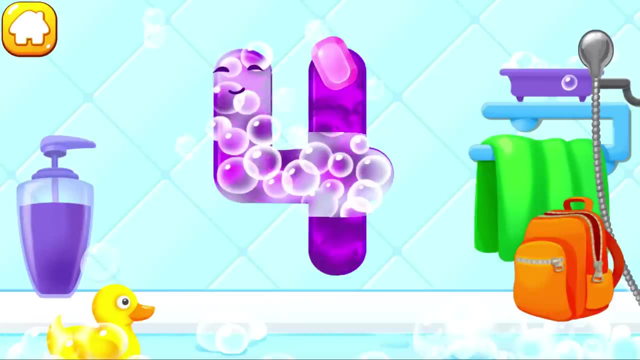 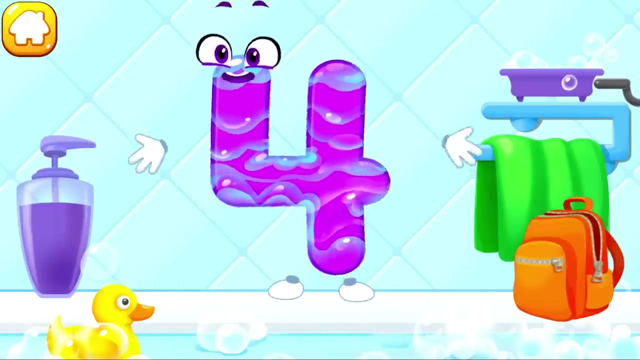 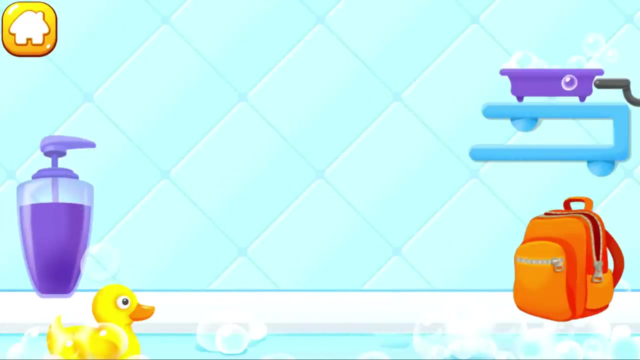 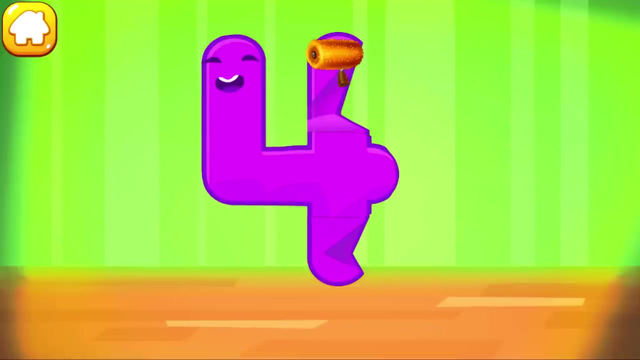 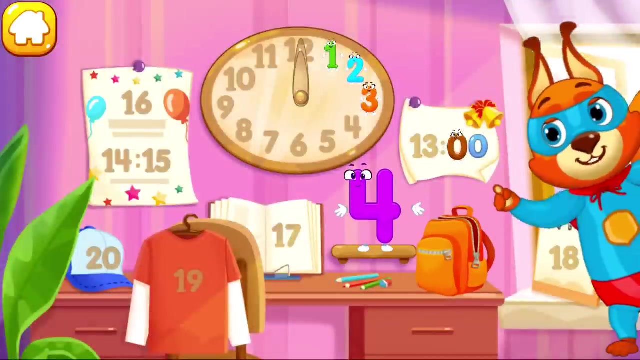 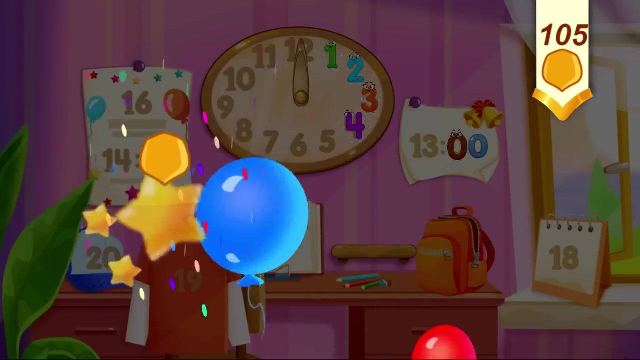 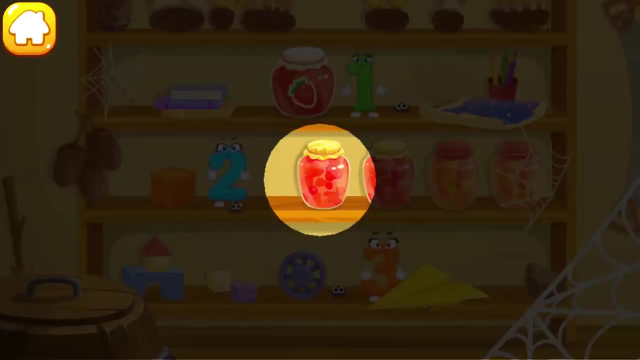 where's number four now? beautiful, wash the number four with soap first. wash away the scope with water. wipe the figure with a towel. you're doing great. iron the number four. good job, put the number four in its place. thanks, you've earned a nut for the squirrel. oh, the nuts got scattered all around the pantry. it's so dark in there. 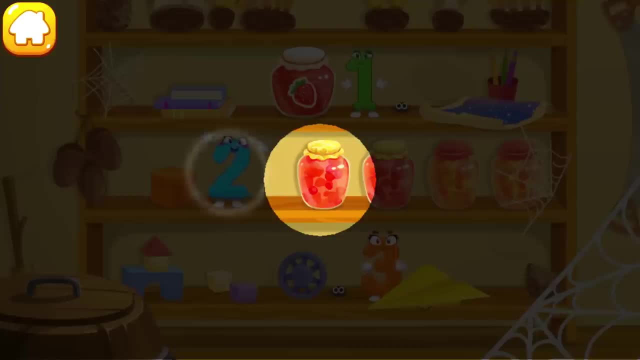 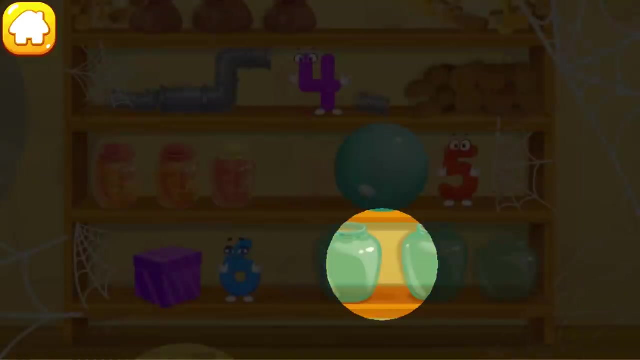 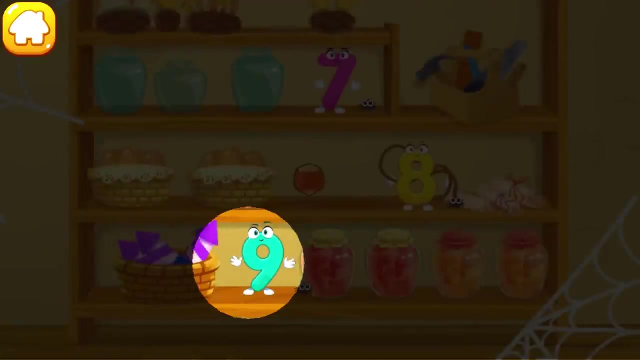 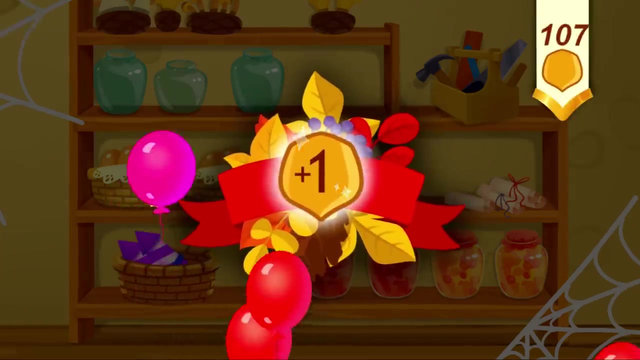 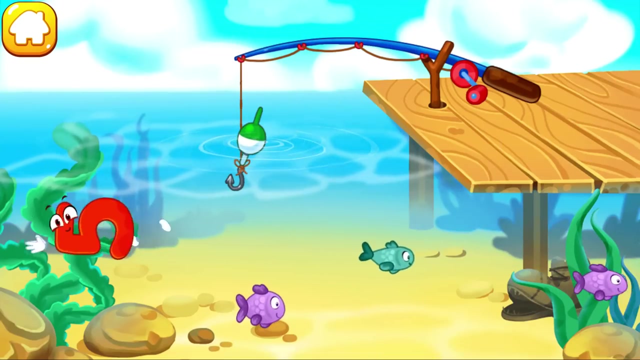 move your finger along the screen to shine a flashlight to the numbers. it's the numbers. they will help us collect all the nuts go on. good, you've earned a nut for the squirrel. the number five flopped into the water and swims with fish. click on the cook to. 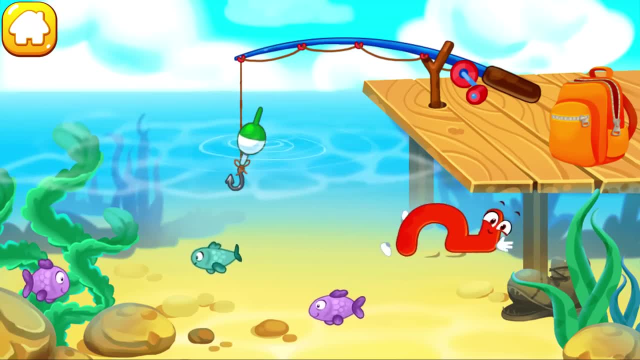 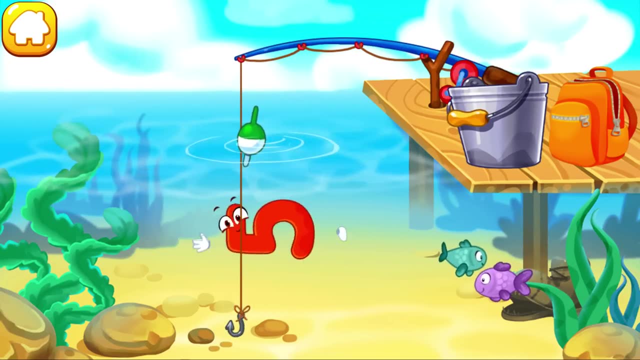 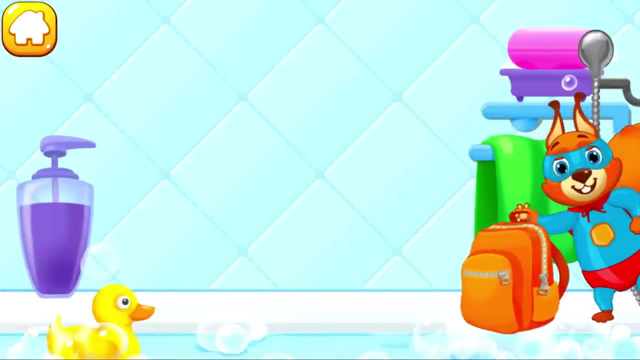 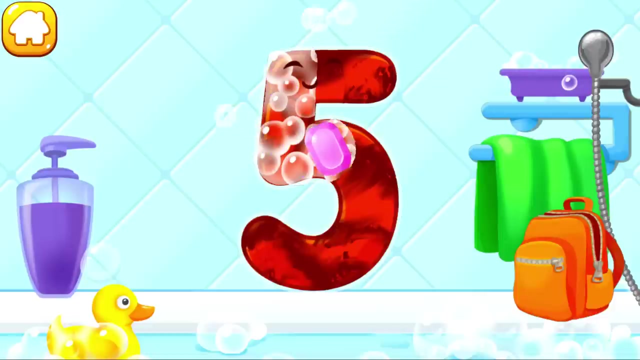 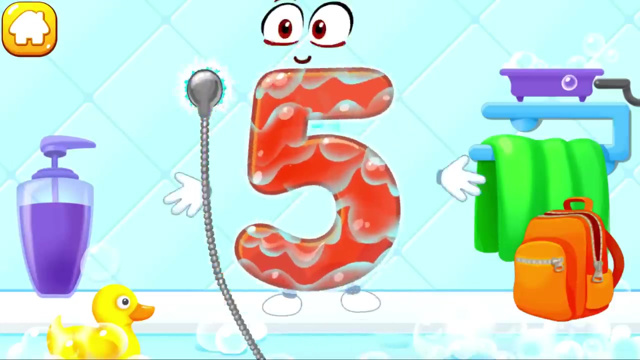 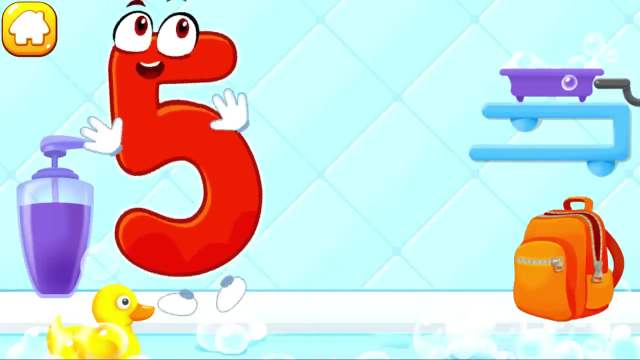 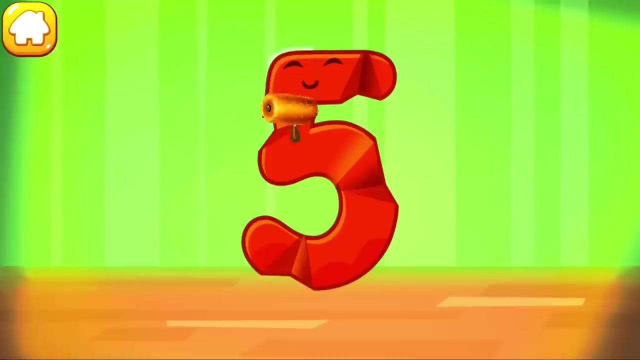 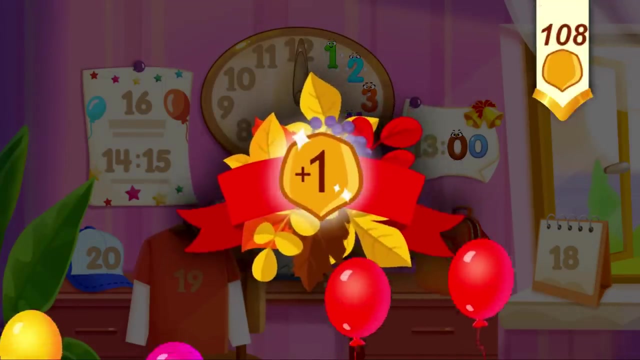 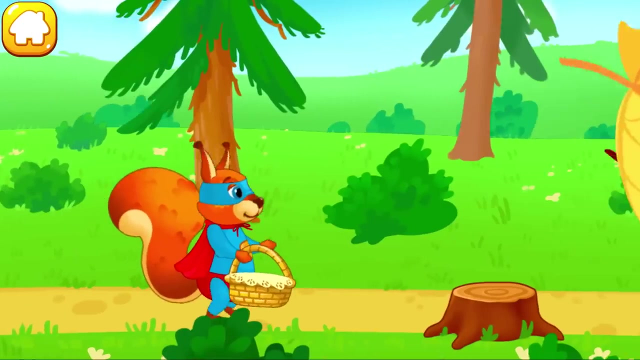 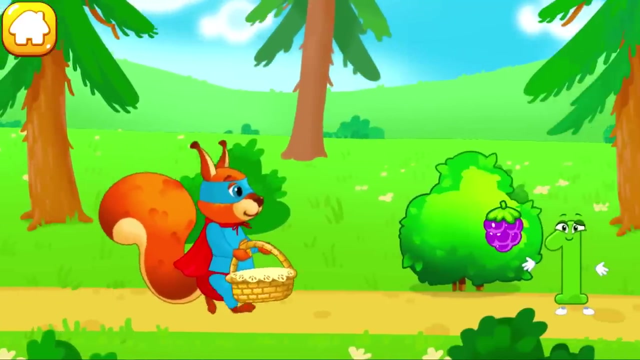 lower it and catch the number or a fish. click the number to pull it out ready. wash the number five with soap first. wash away the soap with water. wipe the figure with a towel. good job, I earned the number five done. put the number five in its place. now I'm safe. take a nut for the squirrel drag. 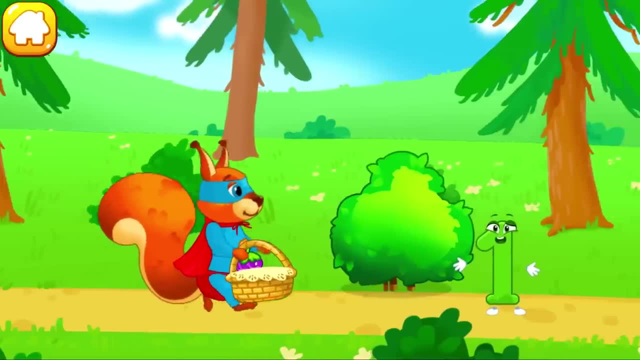 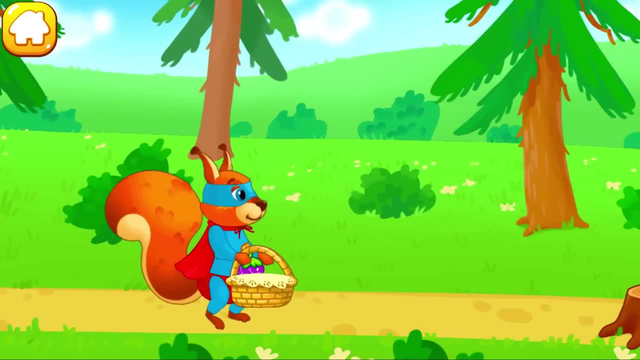 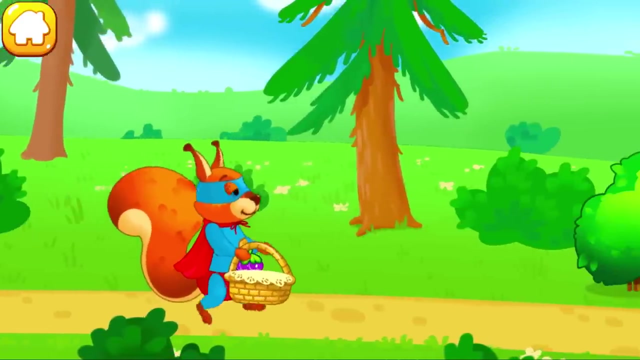 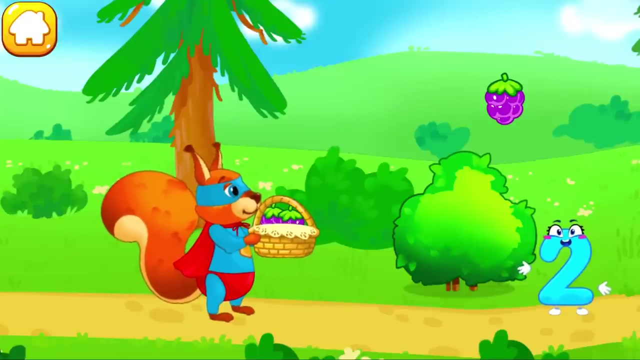 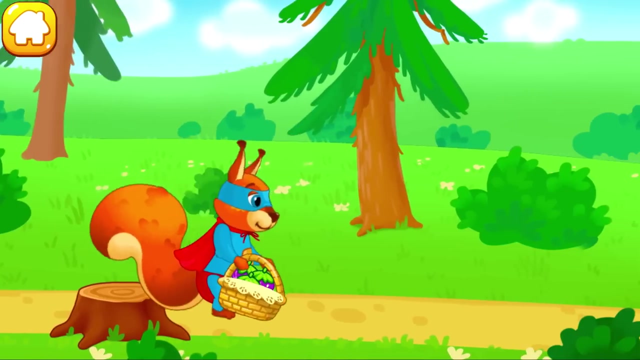 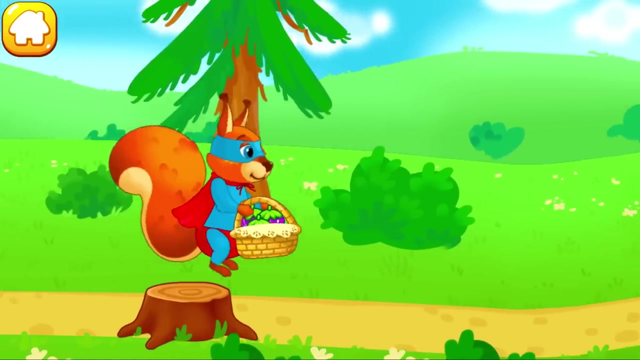 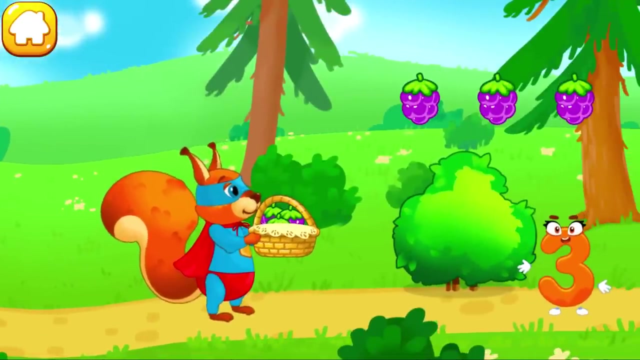 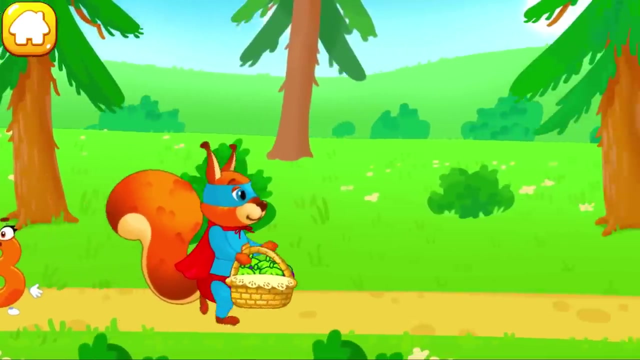 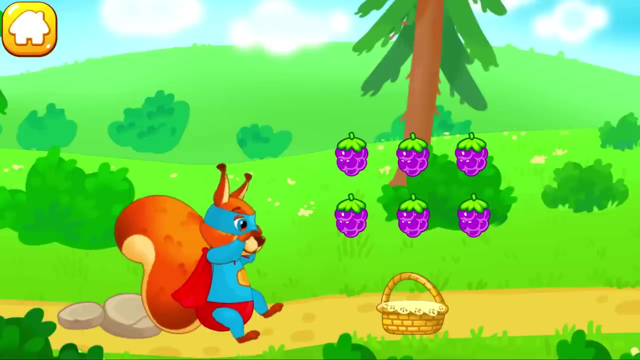 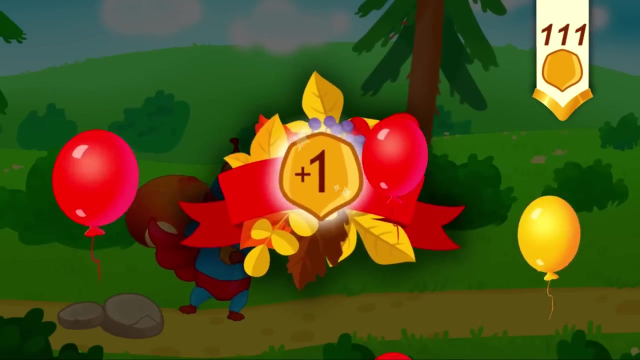 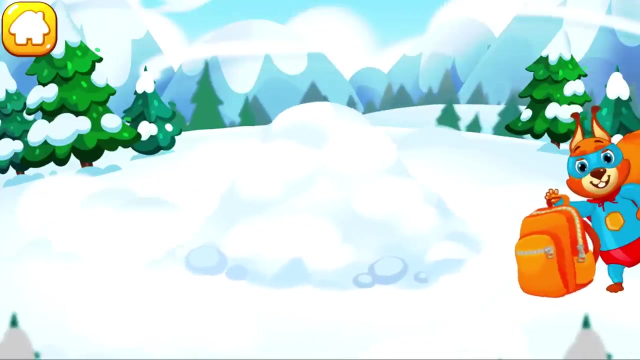 berries into the basket. let's collect more. drag berries into the basket. let's collect more. drag berries into the basket. oh, all the berries got scattered. Drag berries into the basket. Cool, Take a nut for the squirrel. The number six drifted to the mountain's snowy top. 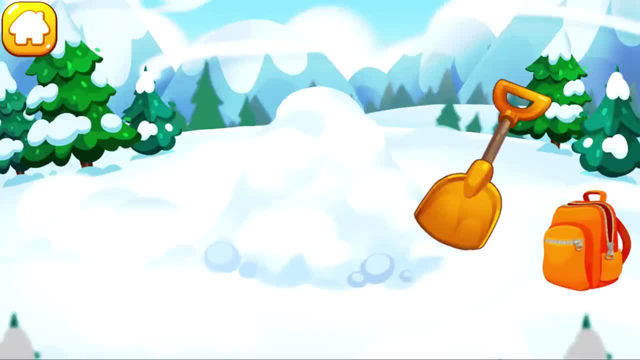 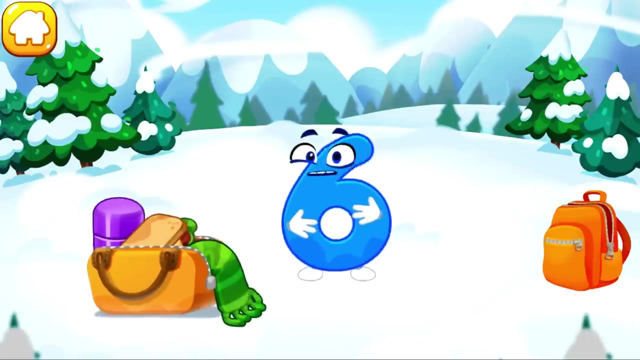 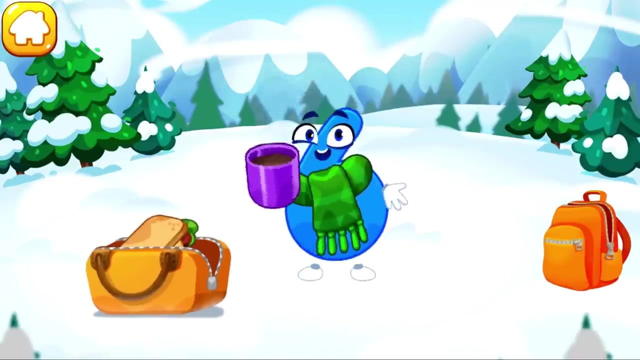 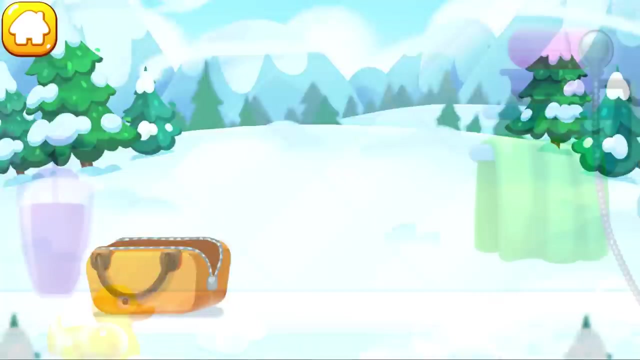 Where is it? In a snowdrift? Let's dig it out. Tap the snow pile. The number six is freezing. Dress her in dry clothes, drink and feed her Ready. Wash- the number six First. apply the snow. 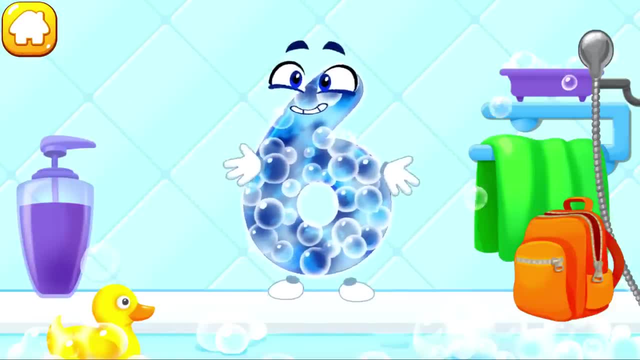 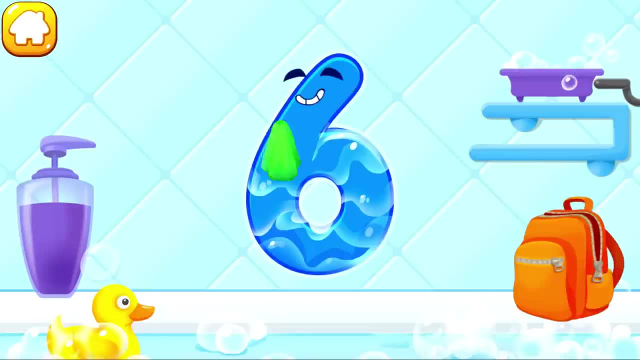 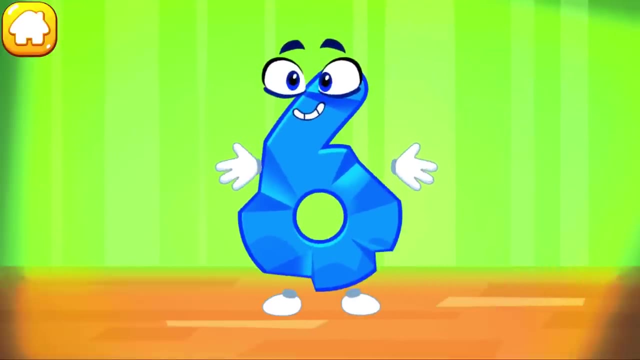 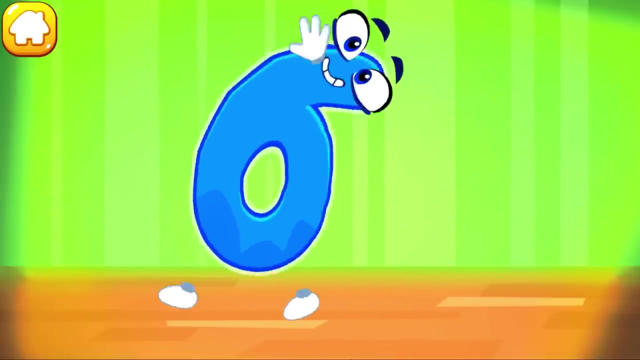 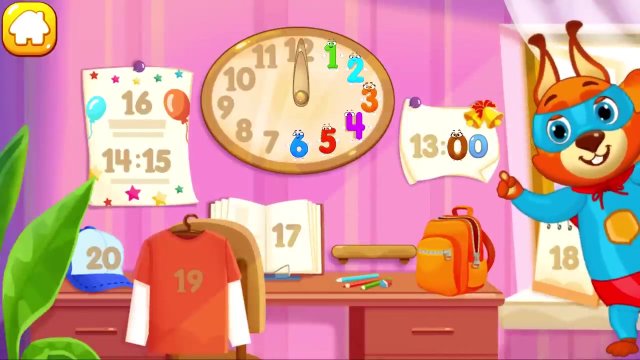 Then apply soap on a number, Wash away the soap with water, Wipe the figure with a towel. Beautiful Iron the number six, Cool, Cool. Put the number six in its place. Thanks, Take a nut for the squirrel. 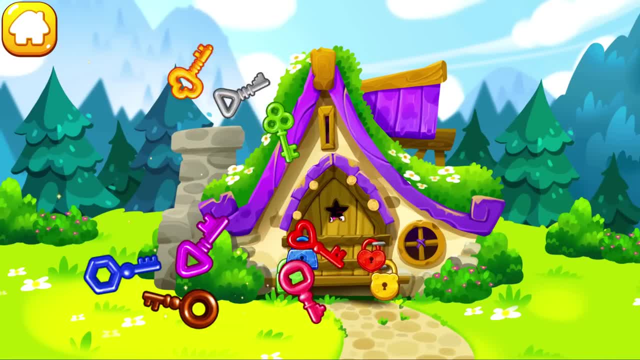 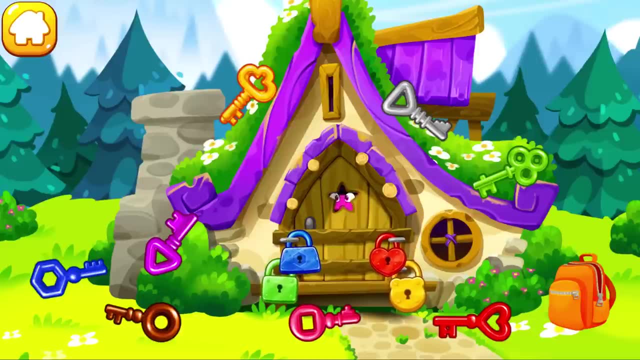 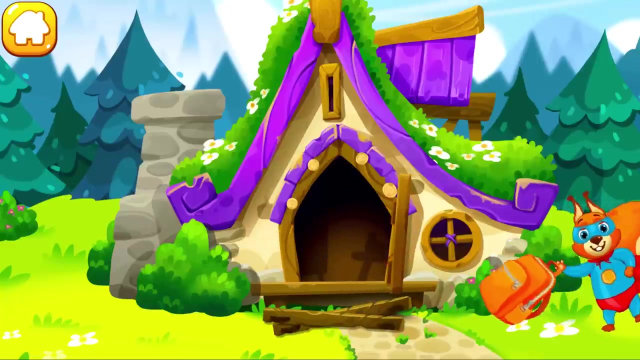 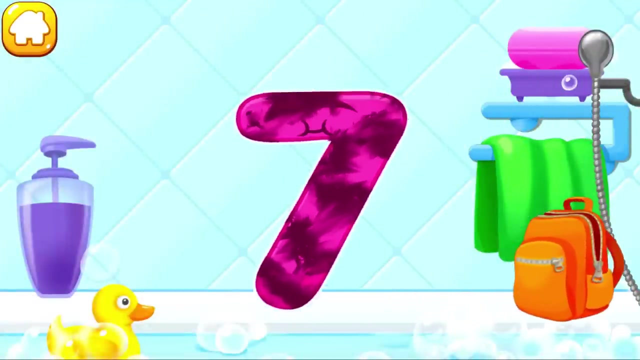 The number seven fell into the hut to the good witch. Unfortunately she's not at home and the door is locked. Help the number to get out. Pick up the key to each lock. Done Wash the number seven With soap first. 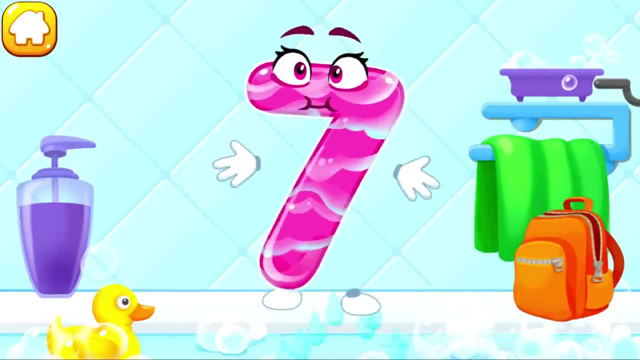 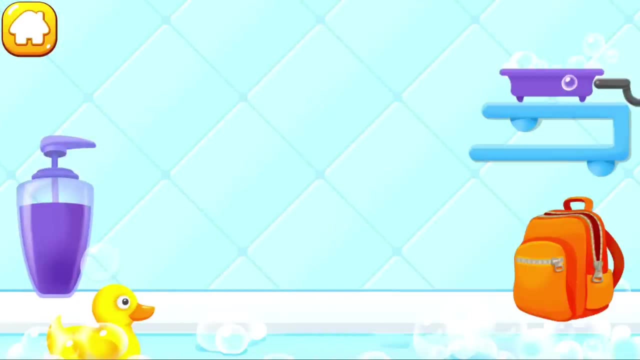 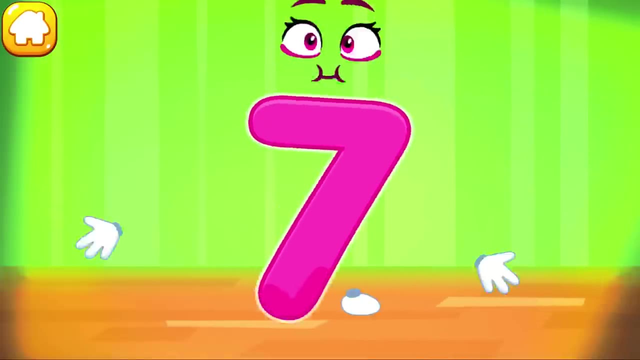 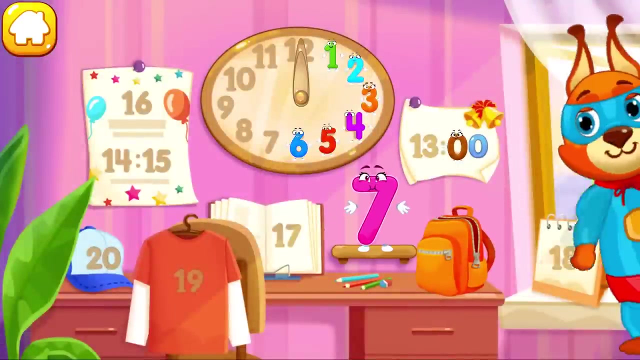 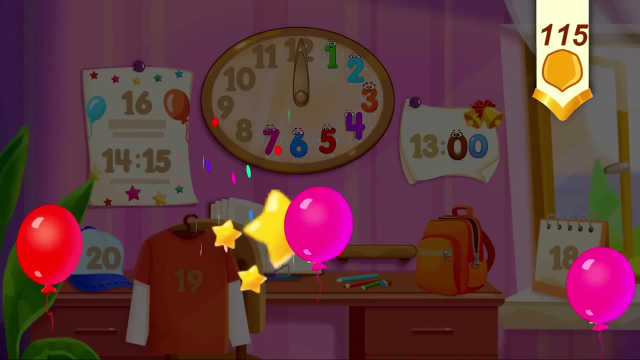 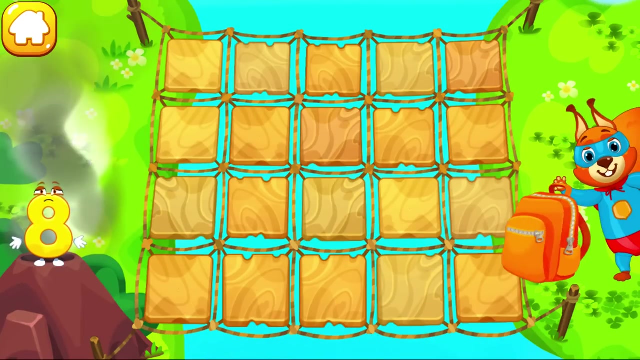 Wash away the soap with water. Wipe the figure with a towel. Good Iron. the number seven: Ready, Put the number seven in its place. Now I'm safe. Take a nut for the squirrel. The number eight hit the smoking volcano. 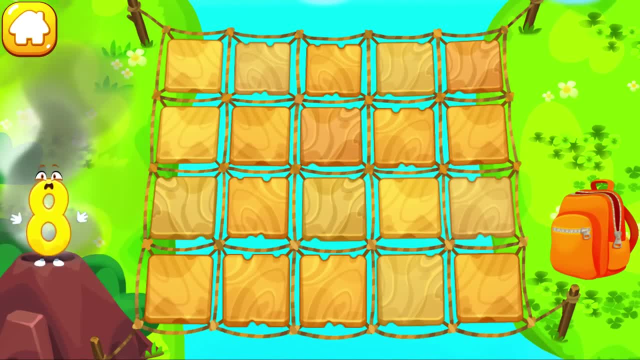 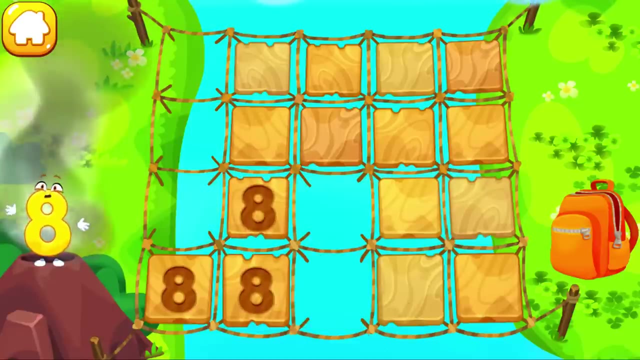 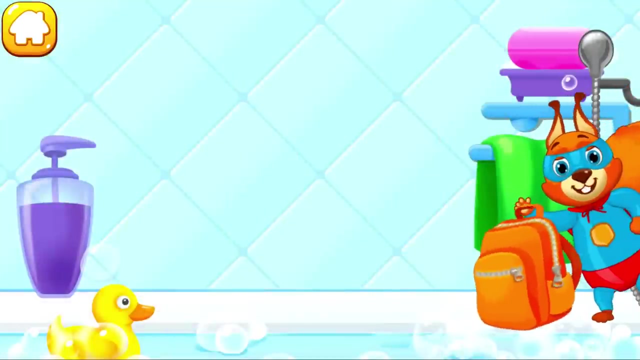 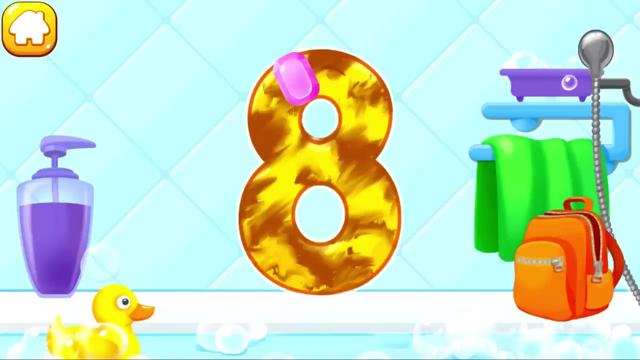 It is hot. Help it cross the bridge. The bridge is old. Some tiles are broken. Click on the tiles. Find a safe way. You're doing great. Watch the number eight. First, apply soap on a number. Wash away the soap with water. 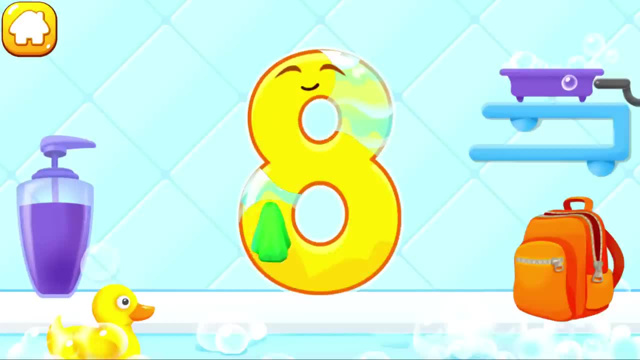 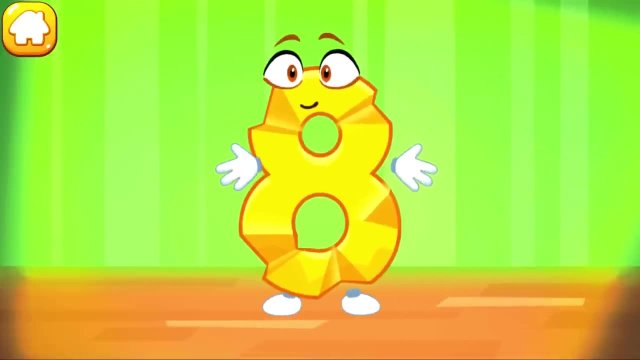 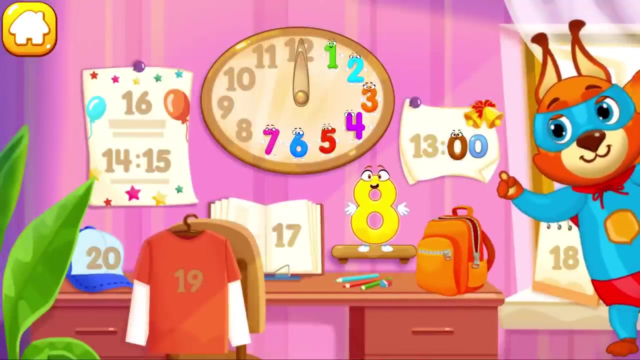 Wipe the figure with a towel Ready. It is hot, Help it cross the bridge. It is hot, Help it cross the bridge. Iron the number eight. Done. Put the number eight in its place. Thanks, Take a nut for the squirrel. 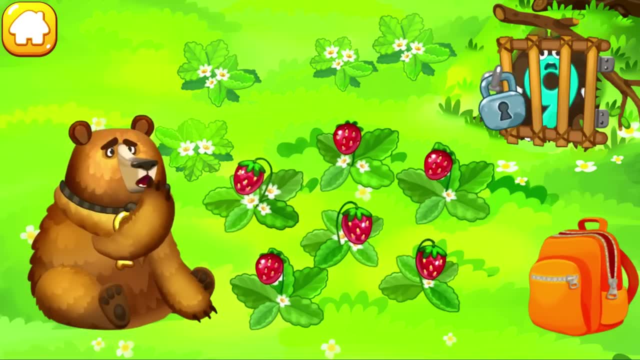 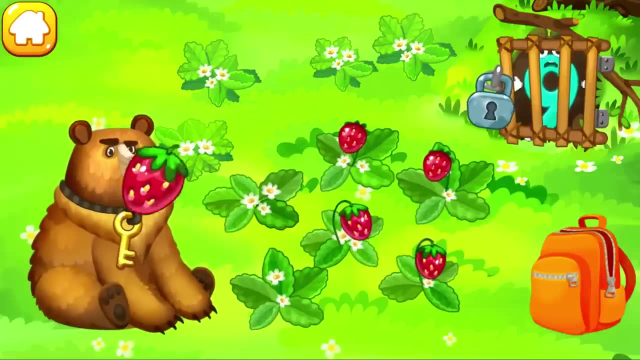 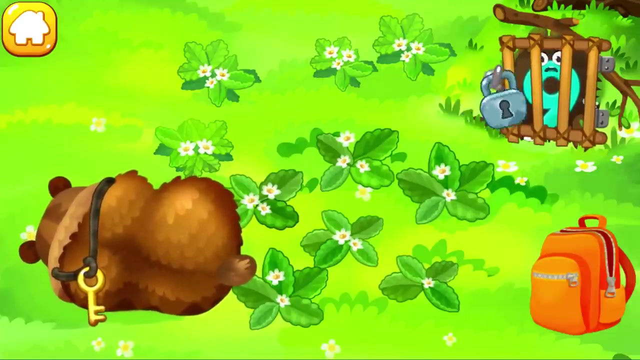 The number nine hit the den of the volcano, den of the hungry bear. feed him with strawberries, maybe he'll fall asleep. drag the berries into the bear's mouth. hooray, and here's the key. open the lock and release the number nine. drag the key. 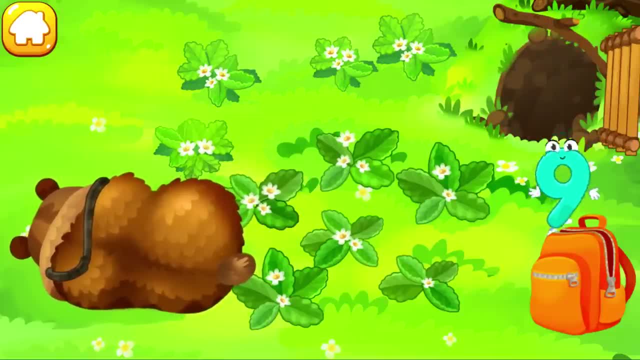 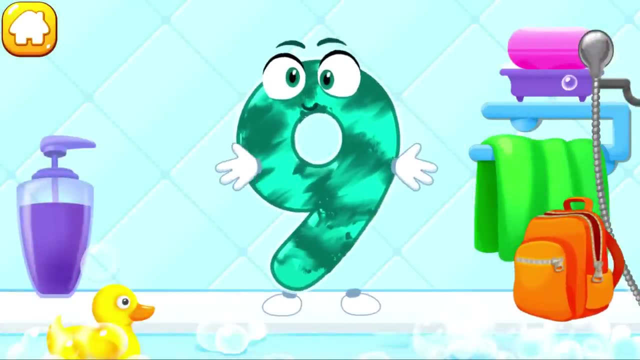 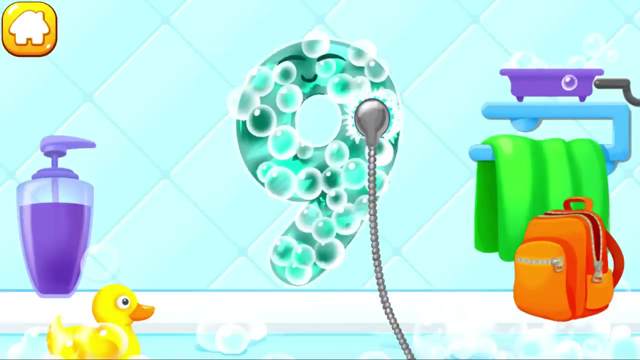 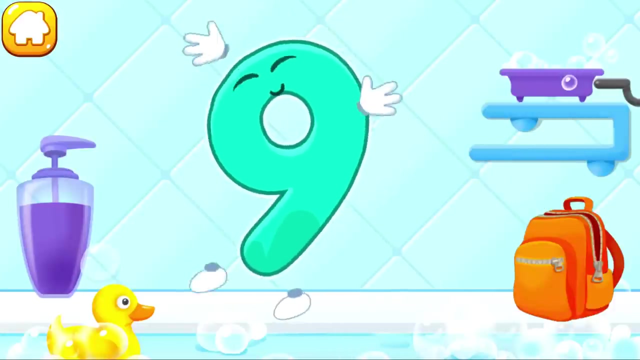 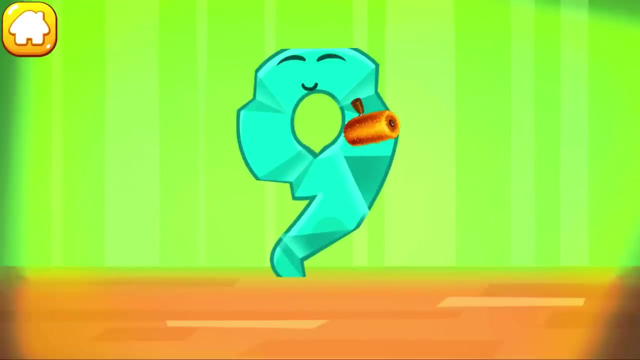 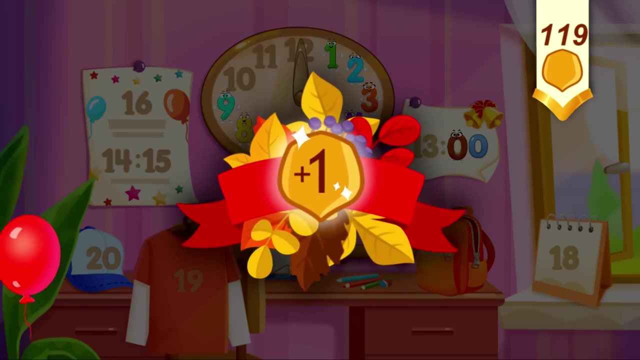 to the lock and the ready. wash the number nine with soap first. wash away the soap with water. wipe the figure with a towel. good job. iron the number nine. done, put the number nine in its place. now I'm safe you've earned a nut for the squirrel. 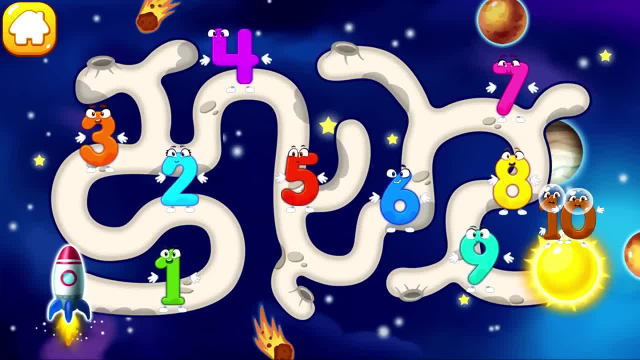 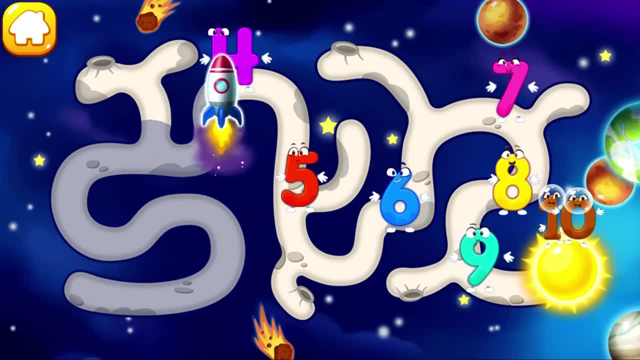 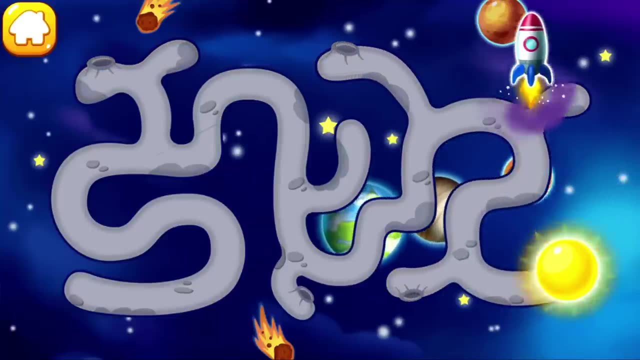 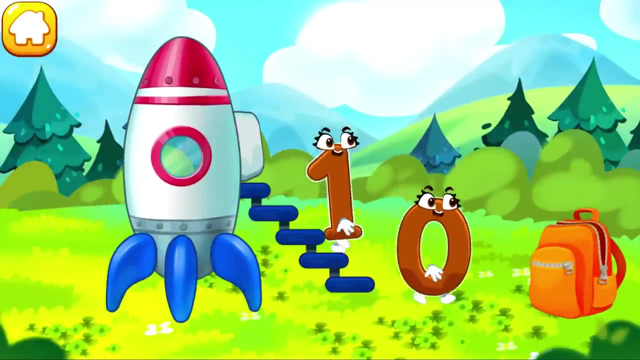 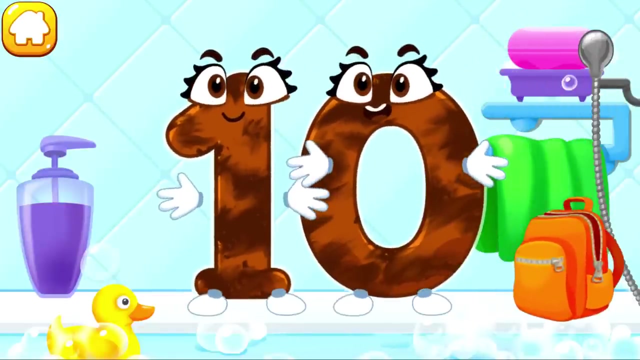 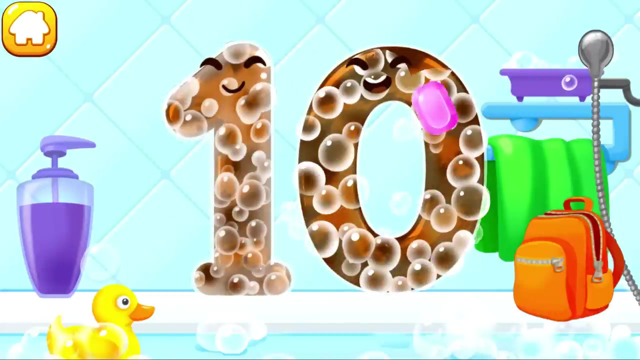 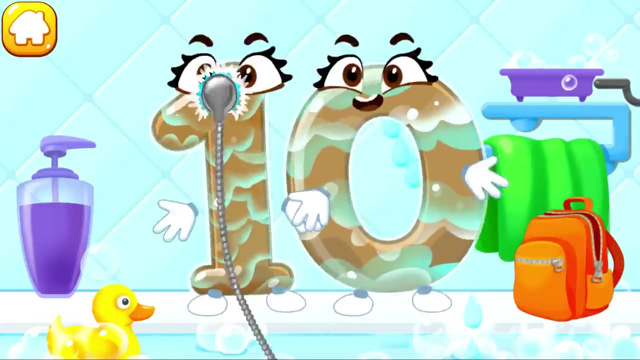 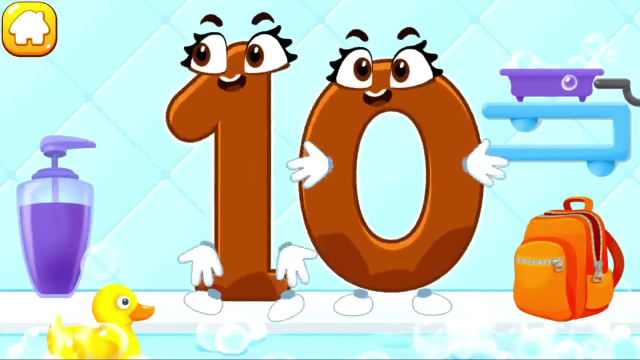 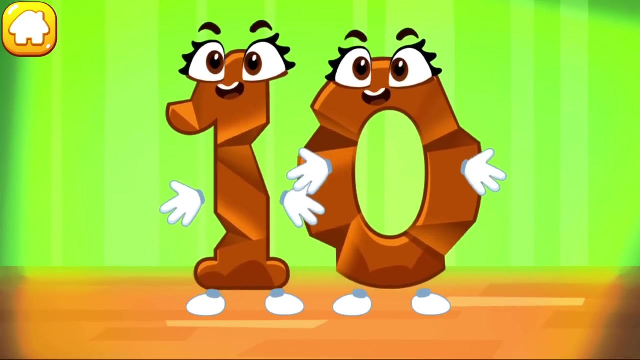 number ten flew right up to the Sun. help the rocket get to number ten. good hooray, number ten has returned to the earth. wash the number ten first. apply soap on a number. wash away the soap with water. wipe the figure with a towel. beautiful, smooth out. 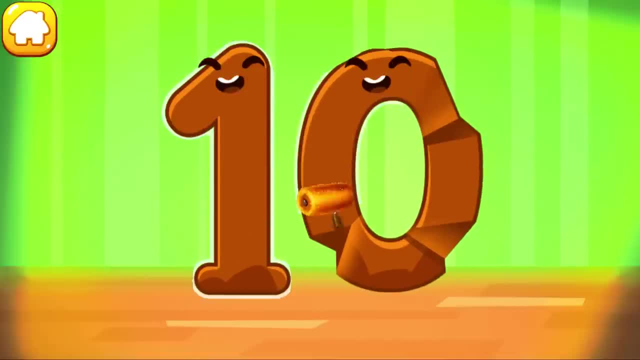 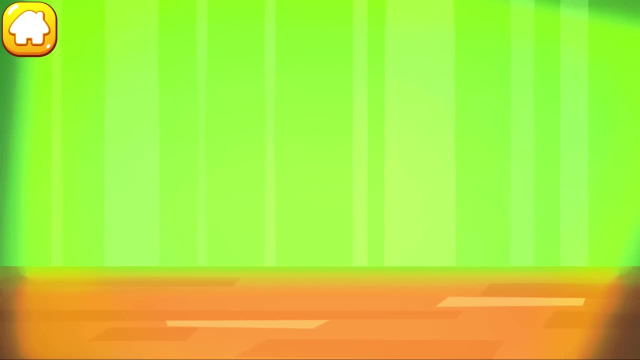 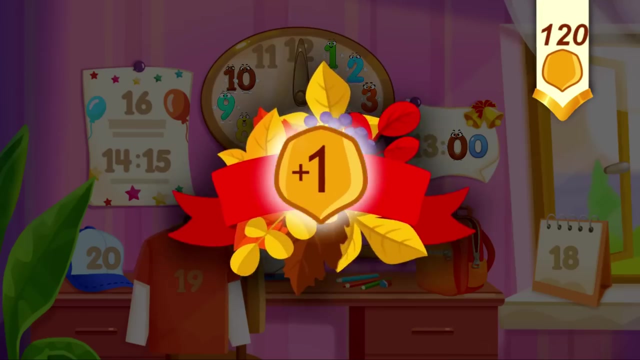 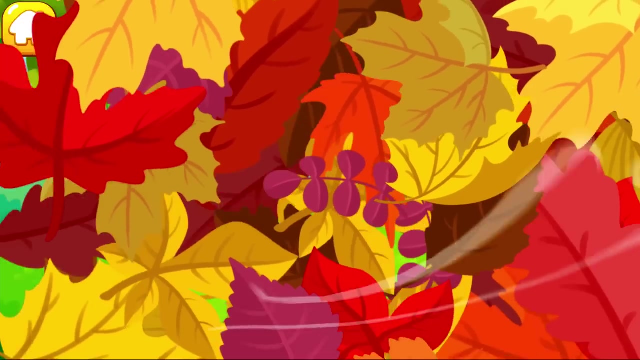 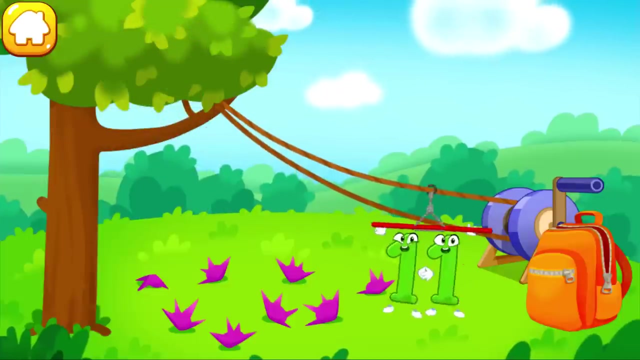 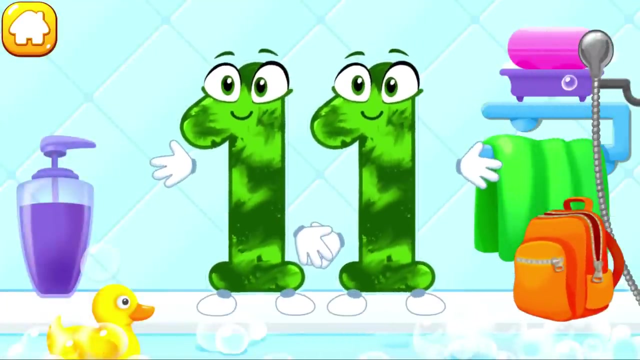 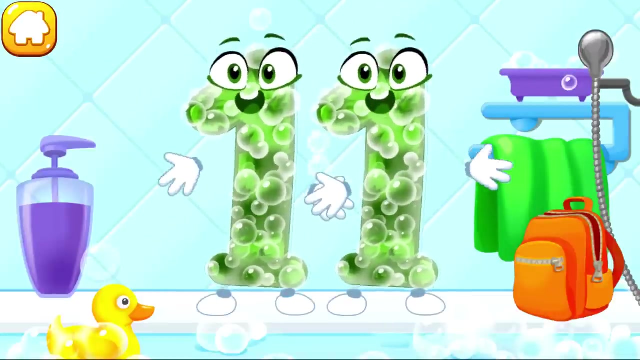 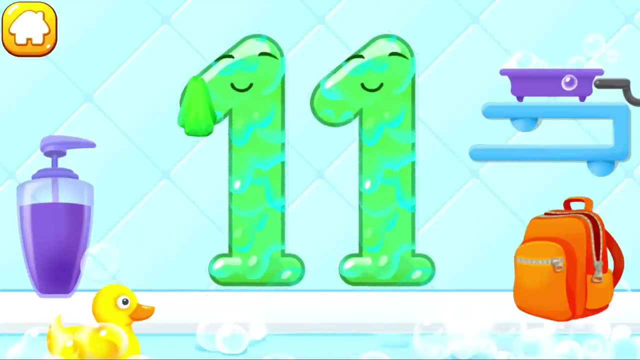 the number ten. good, put the number ten in its place. now I'm safe. you've earned a nut for the squirrel. help number eleven. get down from the tree, throw the handle, got it. wash the number eleven first. apply soap on a number. wash away the soap with water. wipe the figure with. 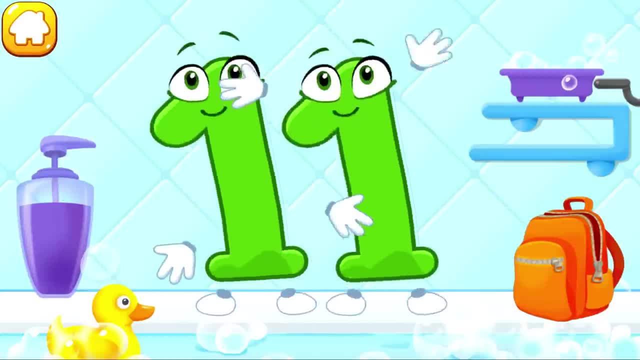 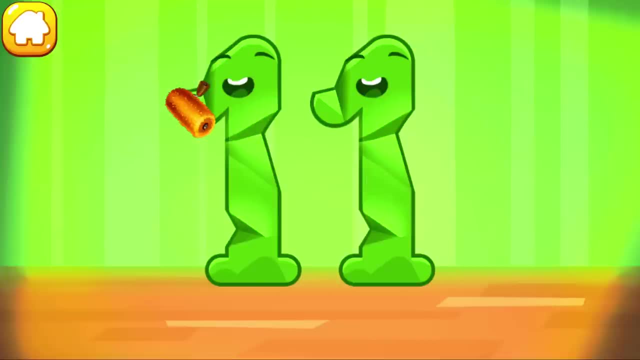 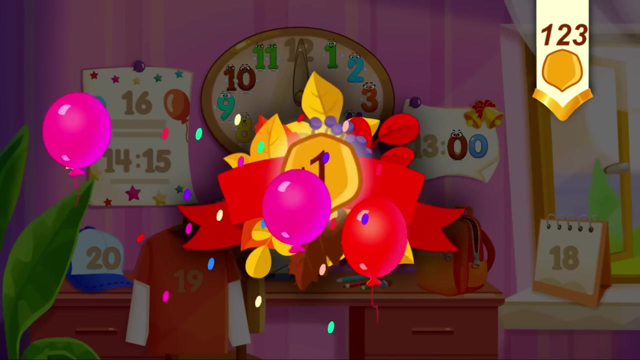 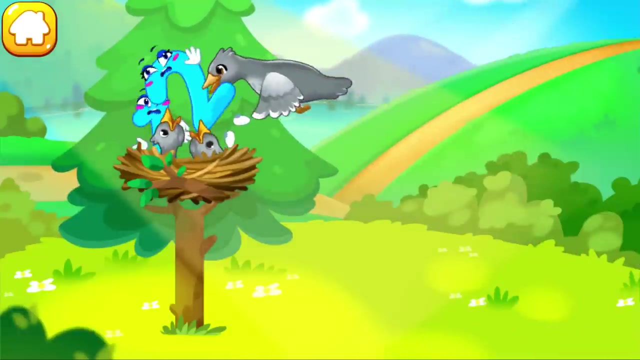 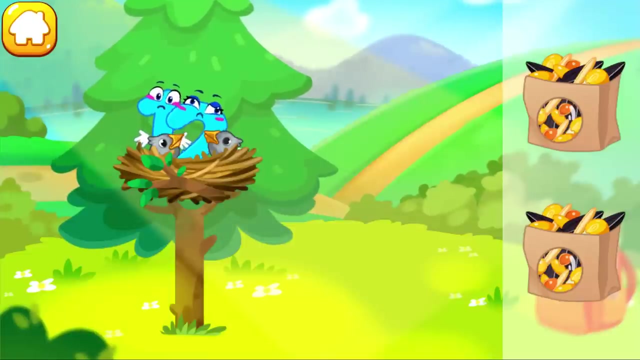 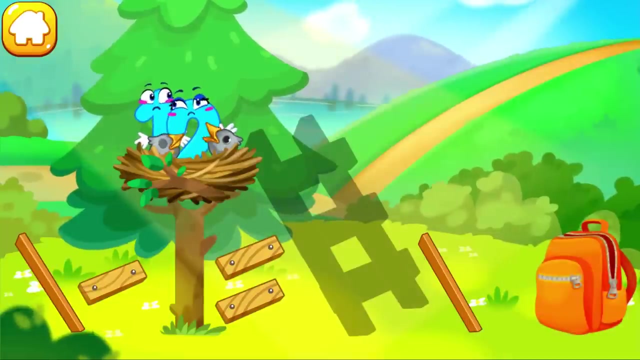 the towel. smooth out the number eleven. good job, put the number eleven in its place. great, you've earned a nut for the squirrel. number twelve got caught by a bird and taken to its nest for the chicks to play with. feed the hungry baby birds with some seeds. now collect the stairs, so 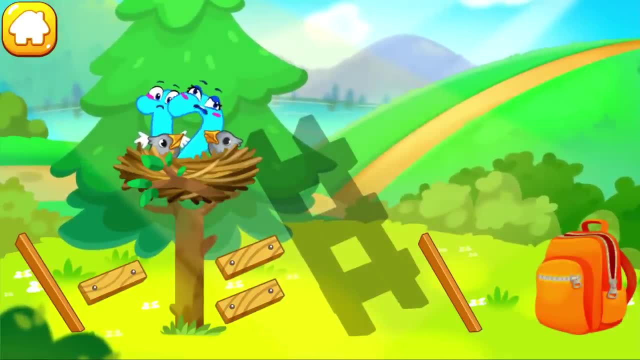 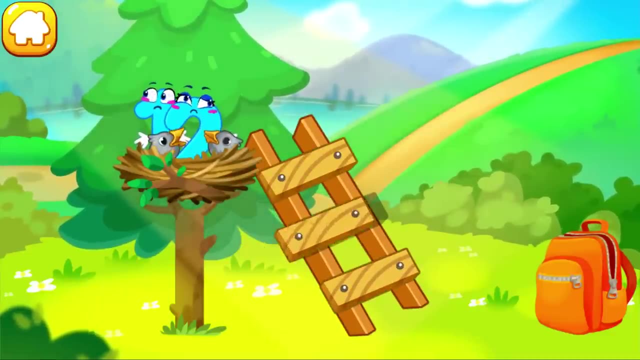 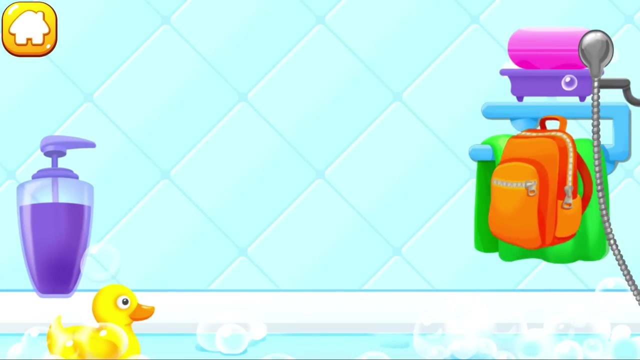 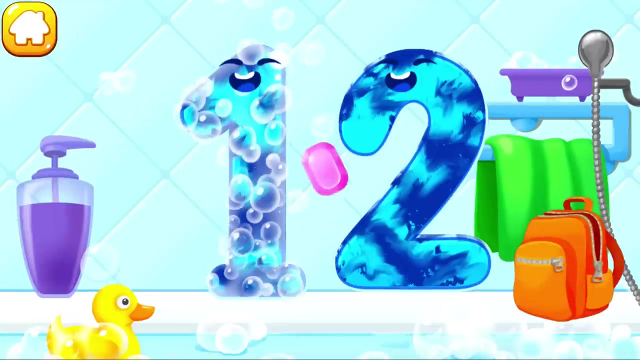 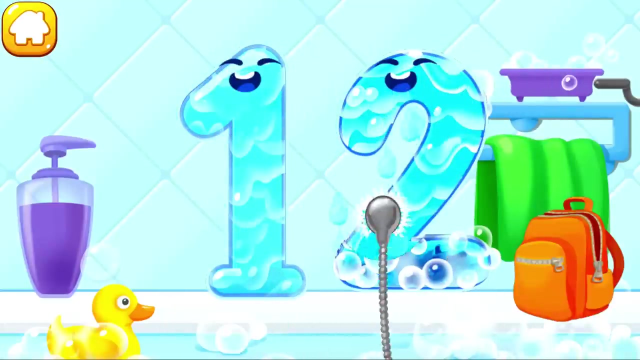 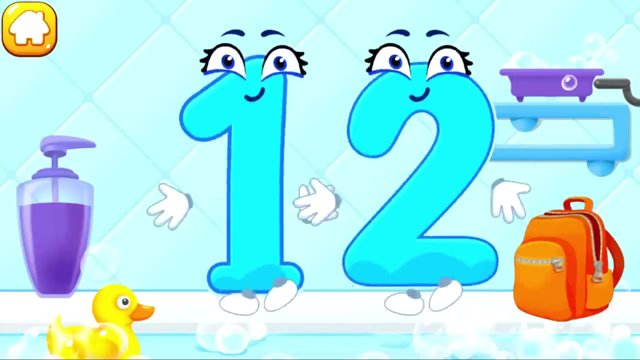 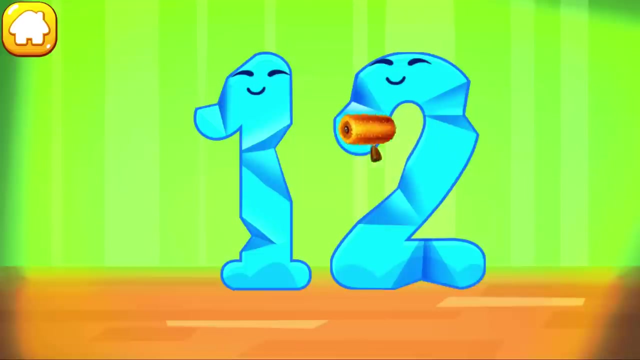 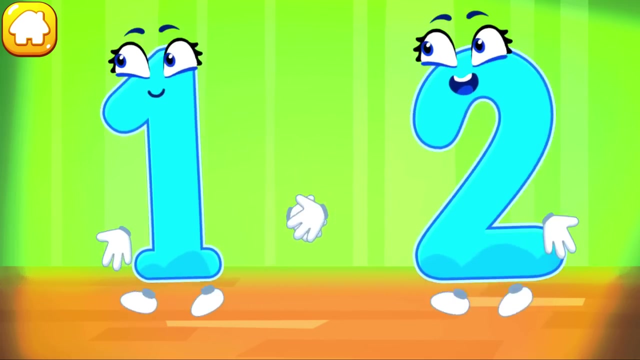 number twelve could get back down. assemble the ladder where it fell apart. wash the number twelve with soap first. wash away the soap with water, water. Wipe the figure with a towel. Done, Smooth out the number twelve. Good, Put the number twelve in its place. 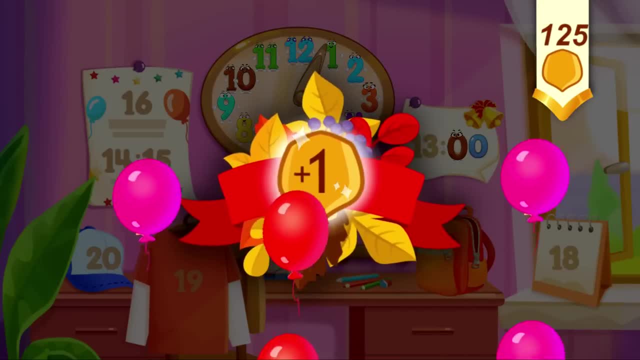 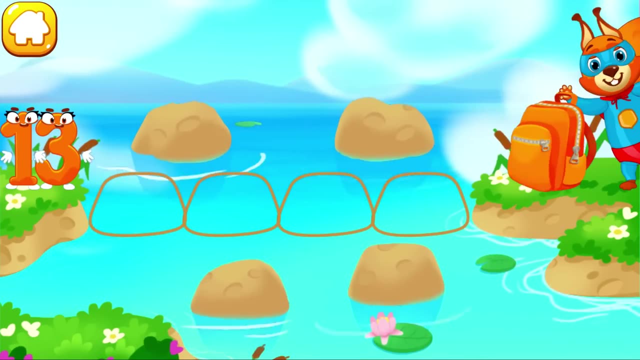 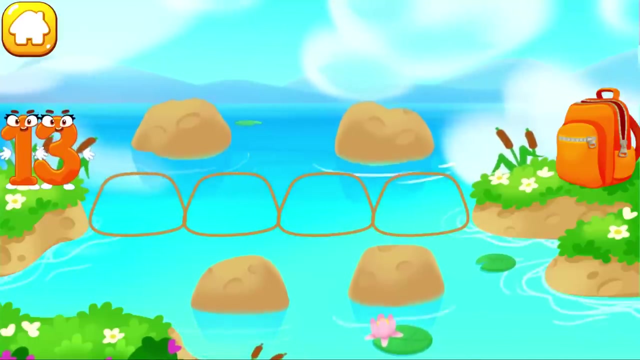 Thanks for the help. Take a nut for the squirrel. Number thirteen found itself on the other bank of the river. Let's make a path from stones so that number thirteen could run over to the backpack. Drag the stones to make a path Cool. 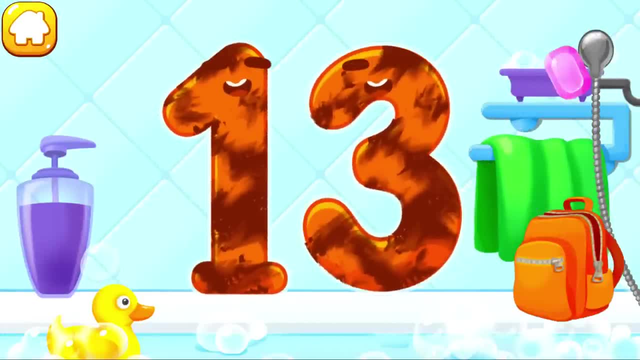 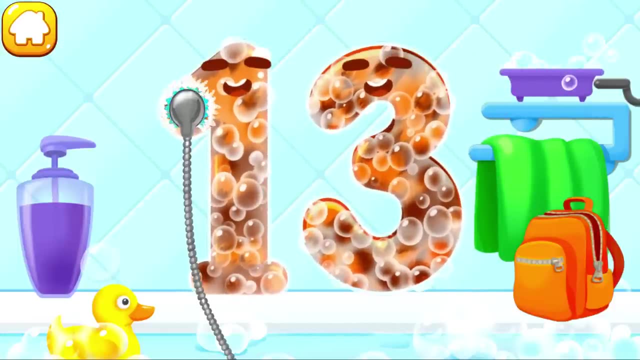 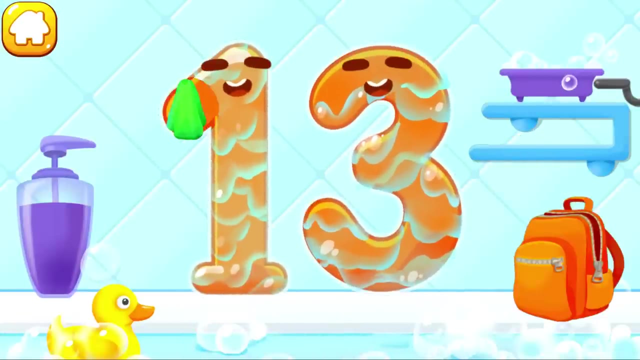 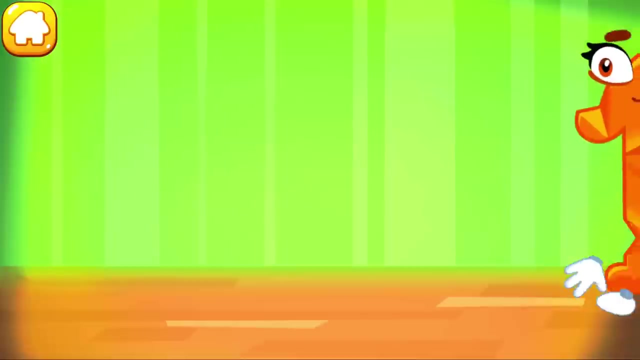 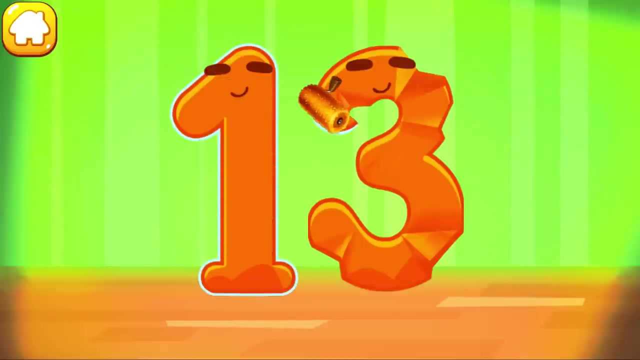 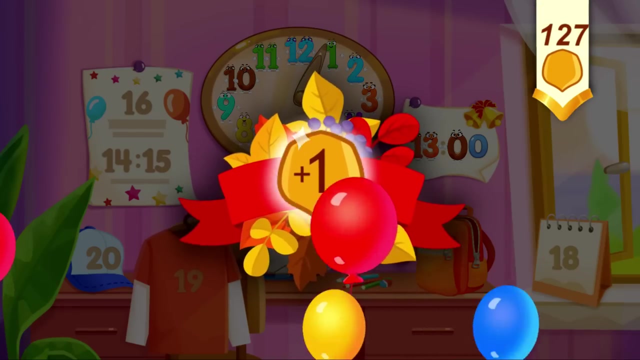 Wash the number thirteen With soap. first, Wash away the soap with water. Wipe the figure with a towel Ready, Smooth out the number thirteen. Good Cool, Put the number thirteen in its place. Thanks for the help. Take a nut for the squirrel. 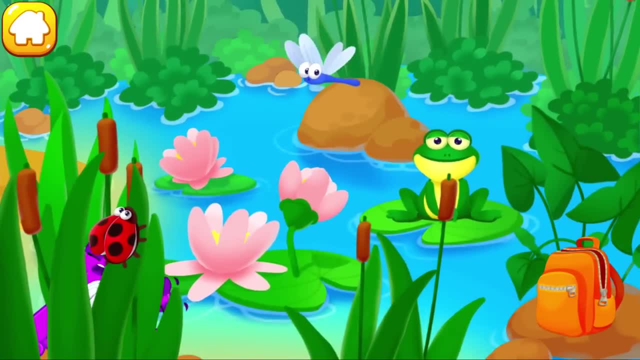 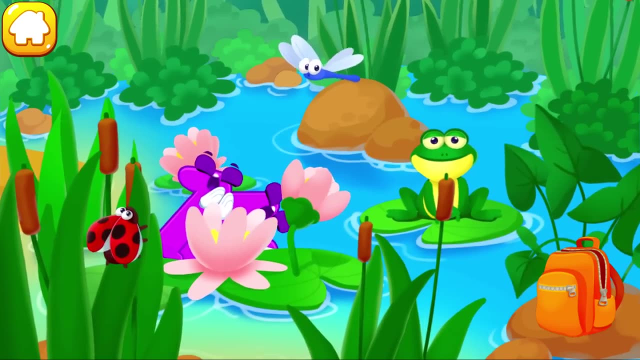 Number fourteen ran into a meadow, got tired and fell asleep. Where's number fourteen now? Number fourteen is playing hide and seek. Let's find it. Where's number fourteen? Let's help the squirrel. Time to find the squirrel Now. 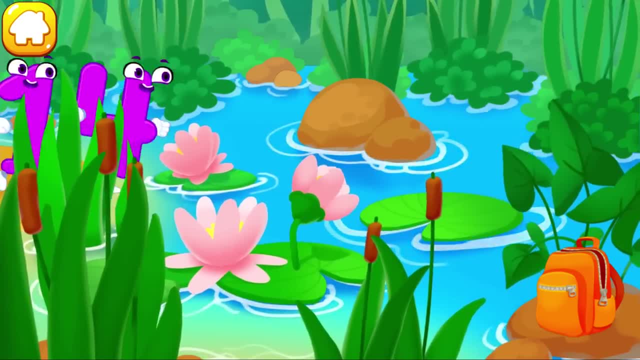 I can't wait to find the squirrel Done Now. the squirrel can run and close the path, But it's too late. Where's number fourteen? We're going to find it now Done. Alright, let's put the squirrel in the water. 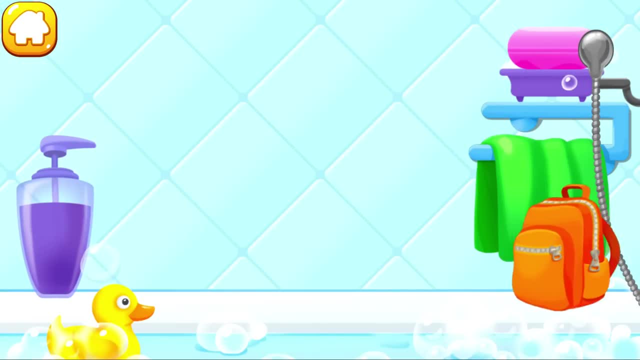 Just like what you did, I'll help the squirrel. That's great, And he's going to find it, And I'll help the squirrel. If I don't find it now, I'll have to take it out. Thank you, squirrels. 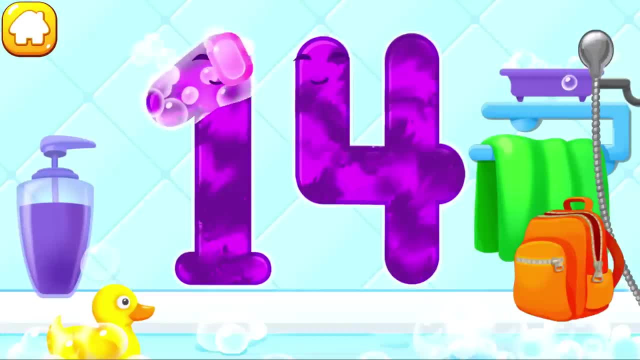 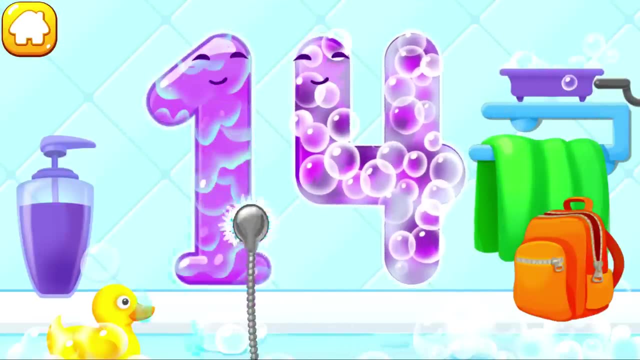 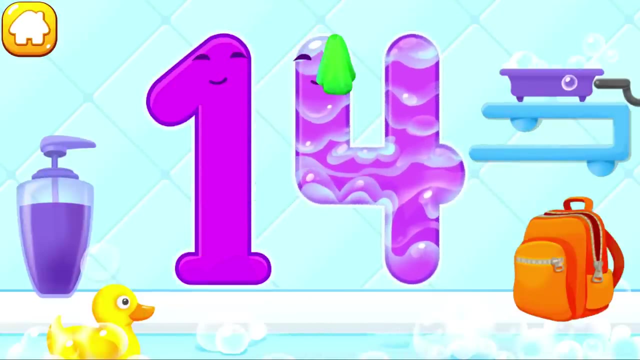 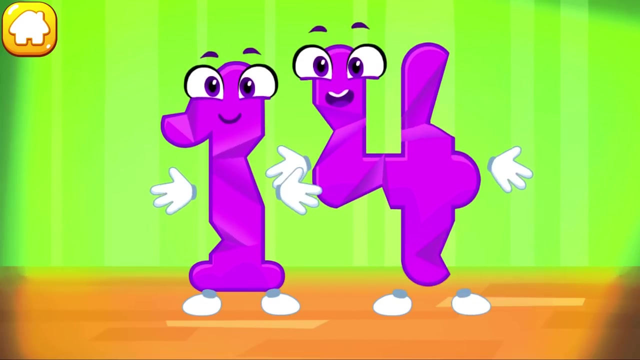 You're very kind, That's what you did for me. Where's number fourteen now Done? Wash the number fourteen First, apply soap on a number First, wash the number fourteen. Wash away the soap with water. the soap with water. wipe the figure with a towel. beautiful, smooth out the number. 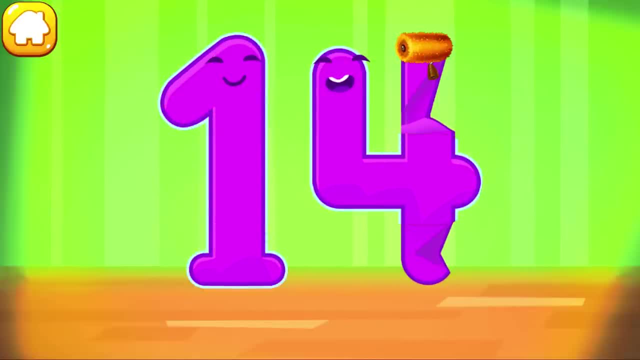 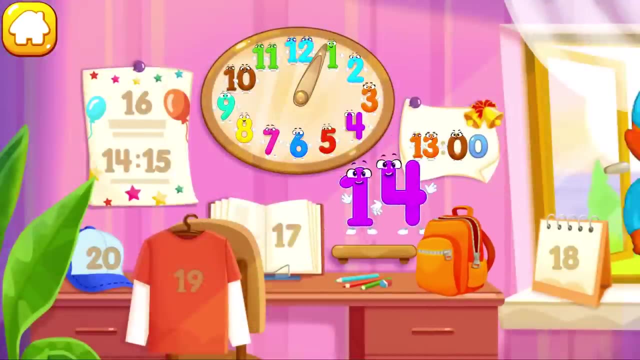 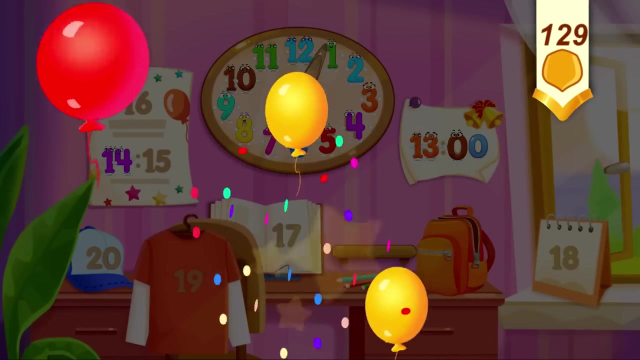 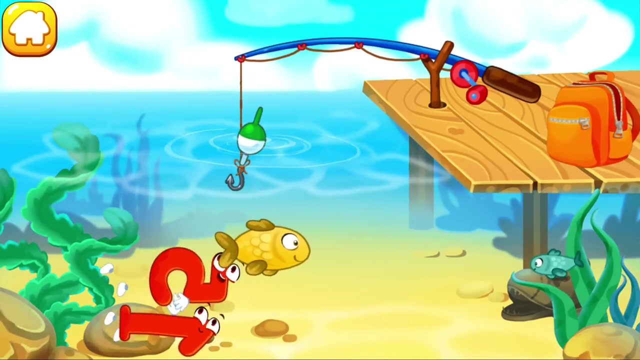 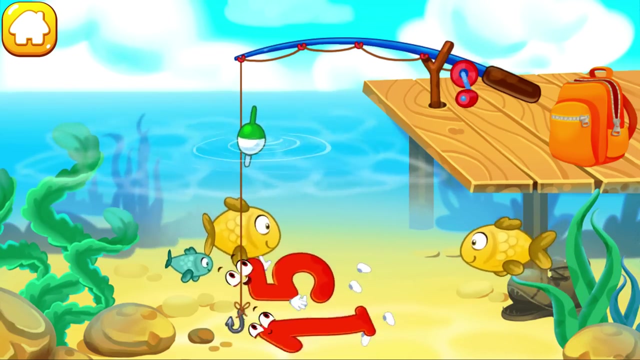 14. good job, put the number 14 in its place. thanks, take a nut for the squirrel. number 15 jumped into the water and is swimming with the fish tap. the fish hook, so it hooks the number, or the fish tee hee. you Tap on the number to pull it out. 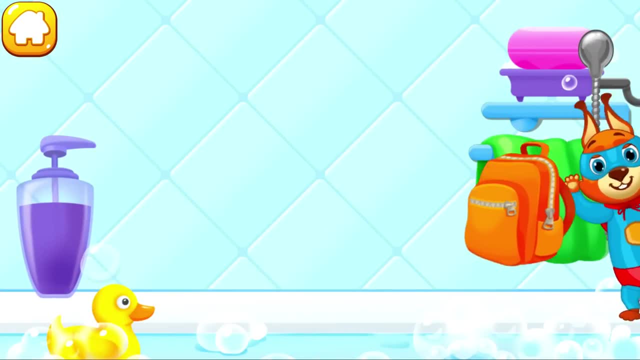 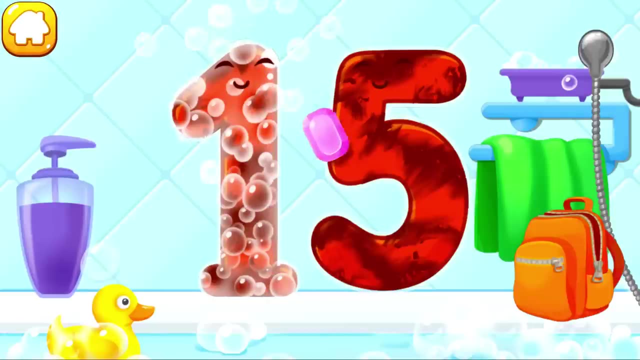 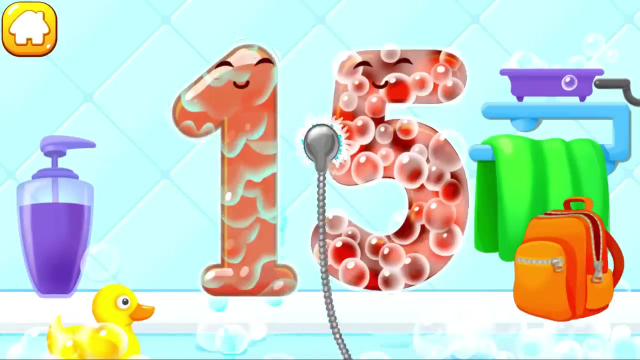 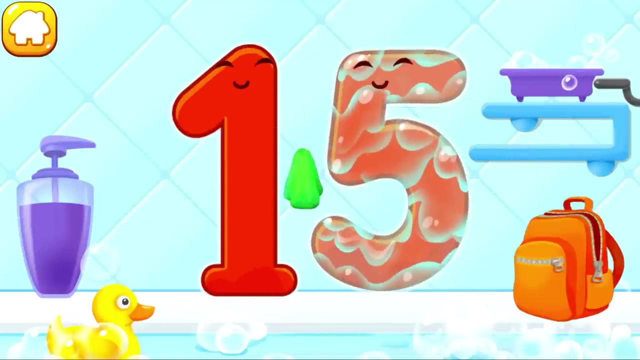 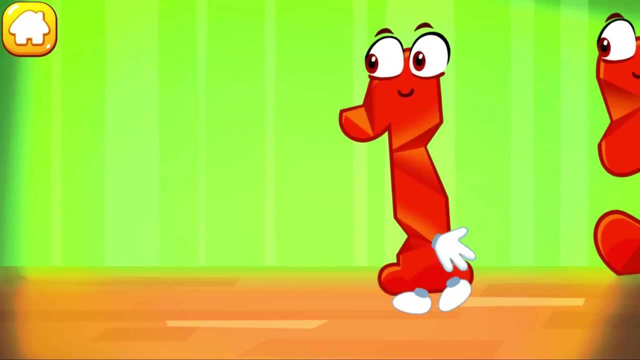 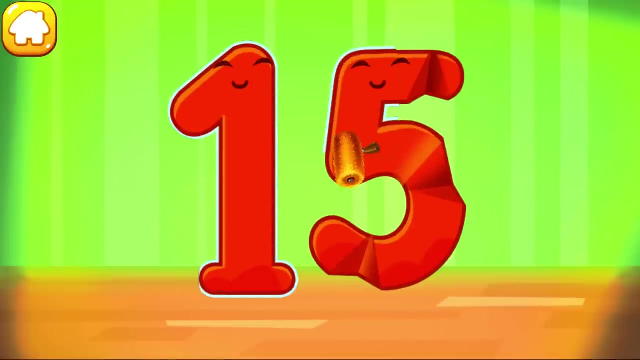 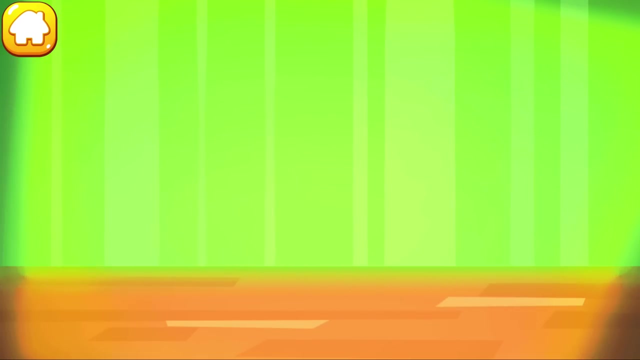 Keep it up. Wash the number fifteen With soap first. Wash away the soap with water. Wipe the figure with a towel. You're doing great. Smooth out the number fifteen. Good job, Put the number fifteen in its place, Great. 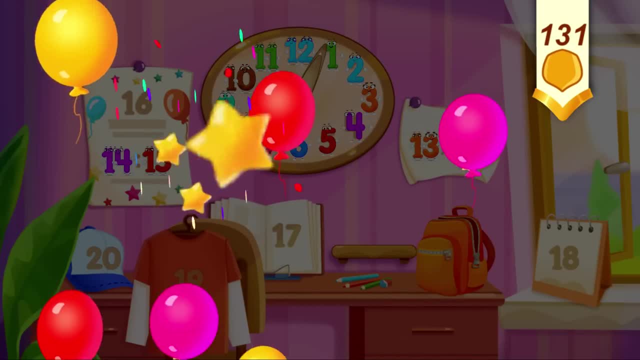 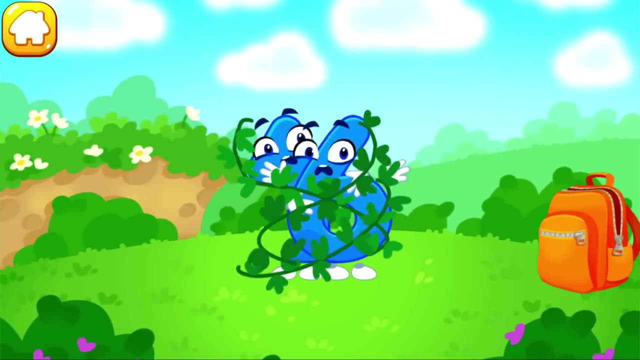 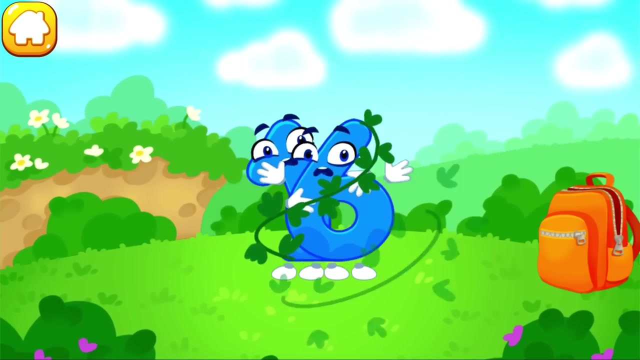 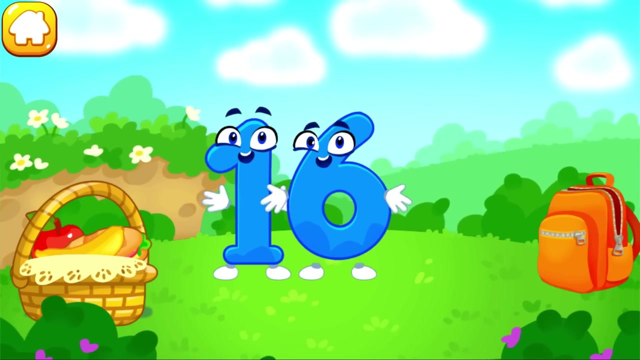 Take a nut for the squirrel. Number sixteen decided to go camping but got tangled up in the twigs. Let's help number sixteen untangle itself. Tap on a twig. Number sixteen got very tired. Let's treat it to something tasty: Tickle, tickle, tickle. 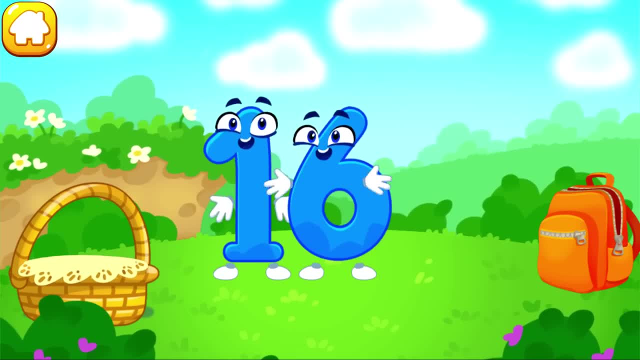 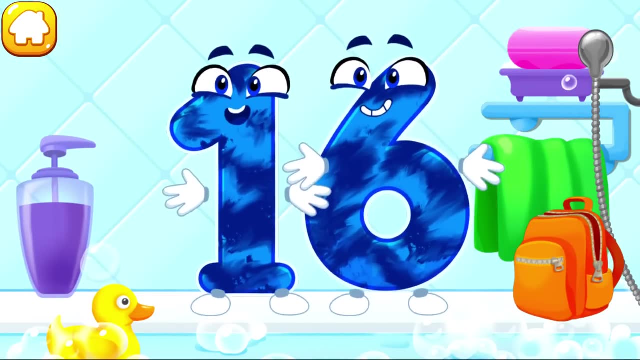 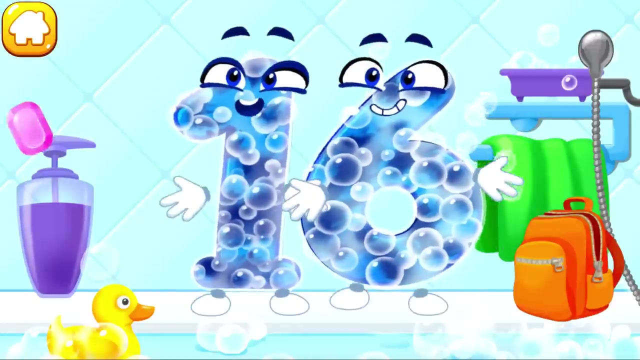 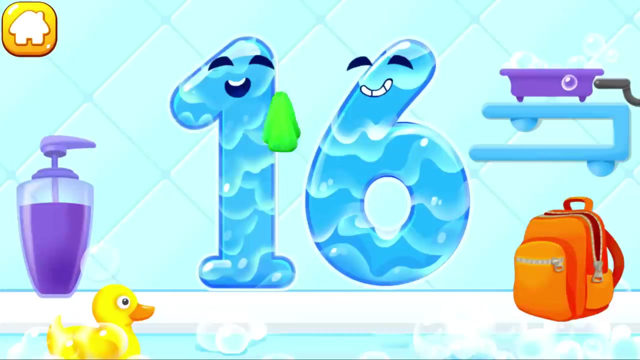 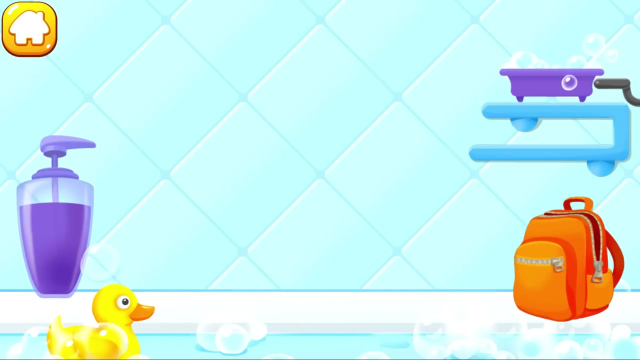 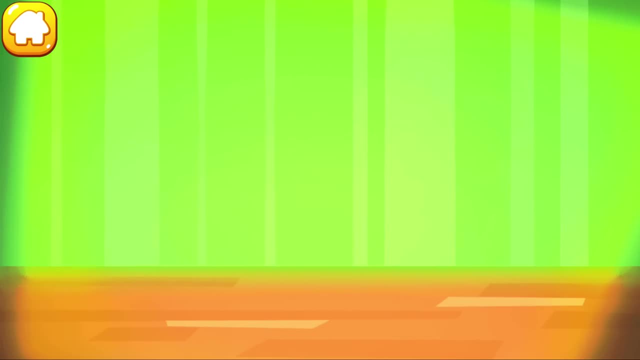 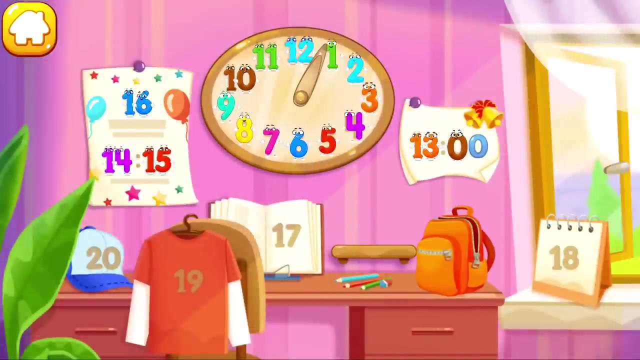 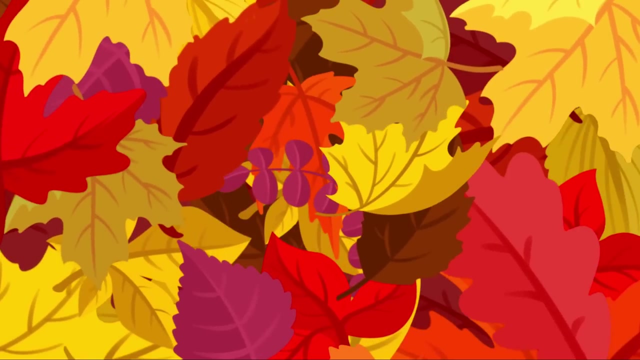 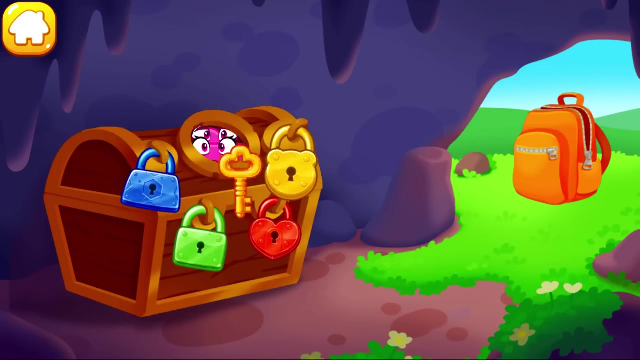 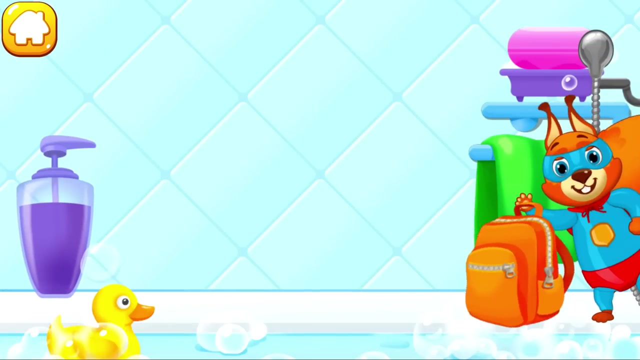 Ready. Put the number sixteen in its place. Now I'm safe. Take a nut for the squirrel. Number seventeen got stuck in a chest. Help the number get out. Find the key for For each lock. Wash the number seventeen With soap first. 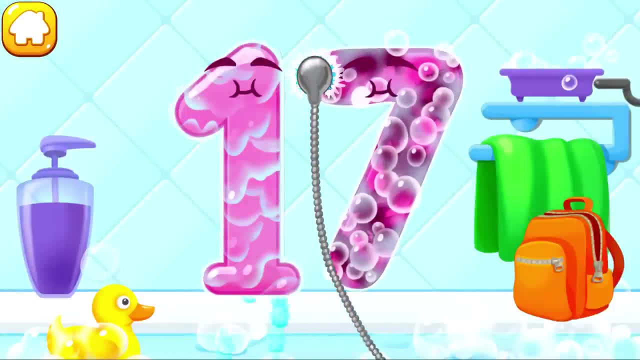 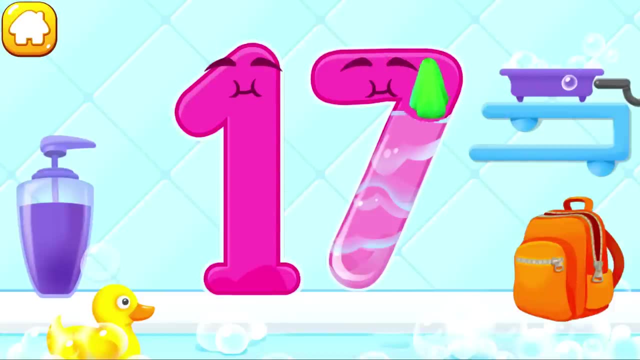 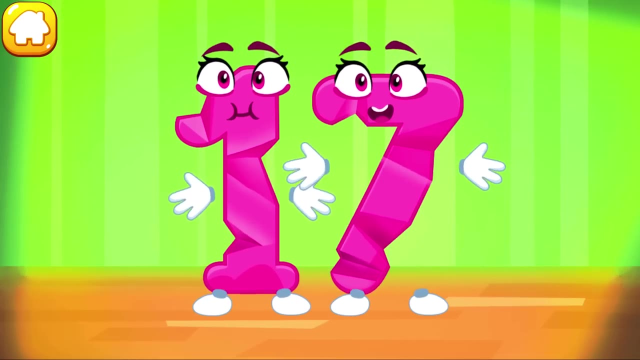 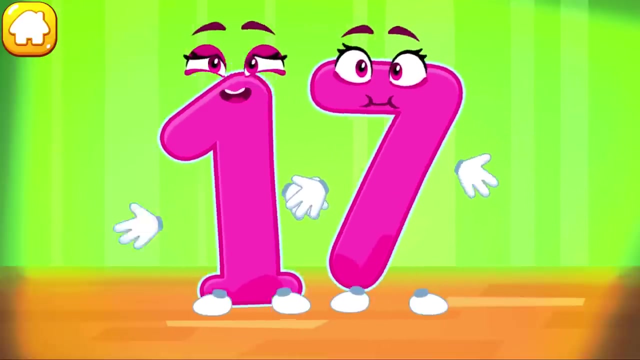 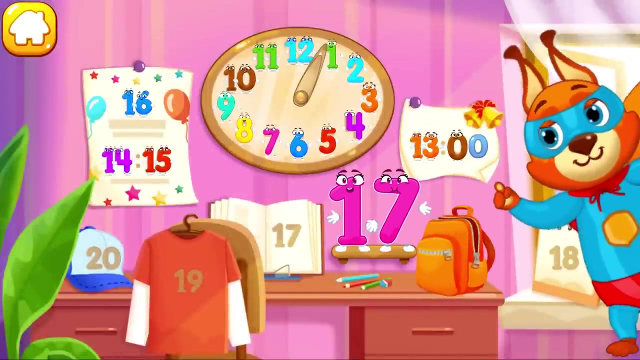 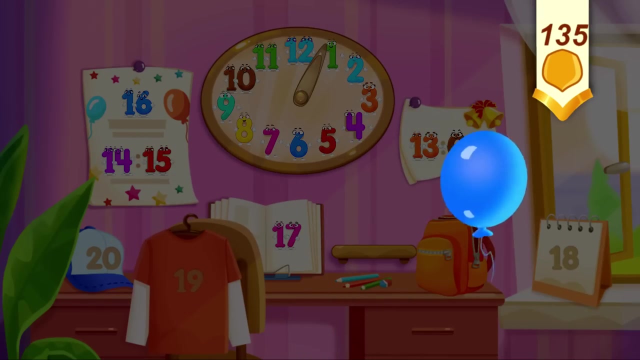 Wash away the soap with water. Wipe the figure with a towel. Good, Smooth out the number seventeen. Good job, Good job. Put the number seventeen in its place. Now I'm safe. Take a nut for the squirrel. Take a nut for the squirrel. 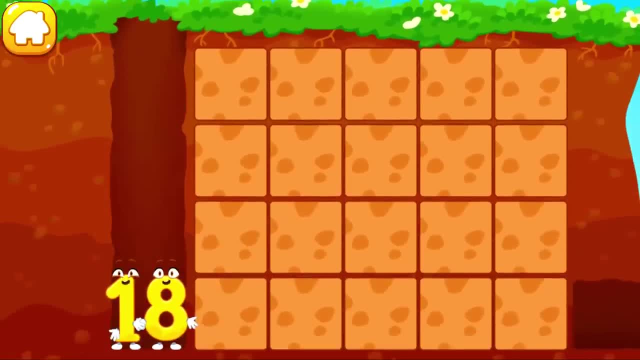 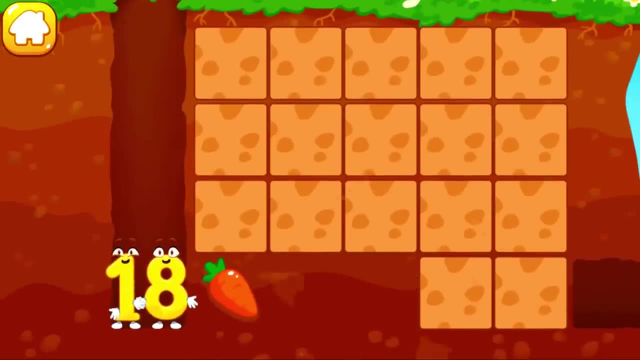 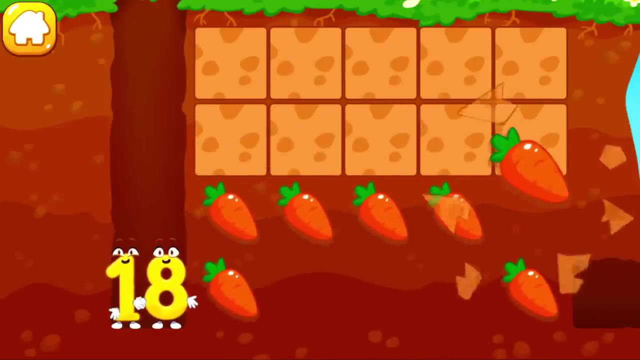 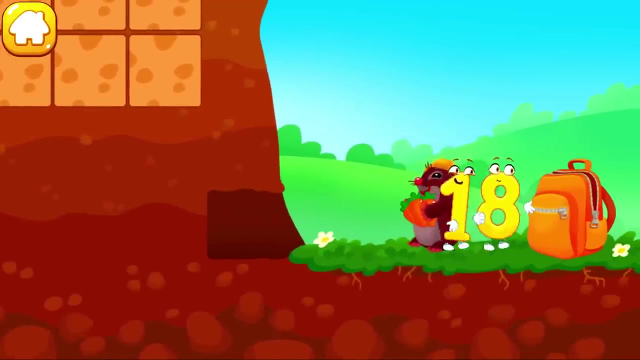 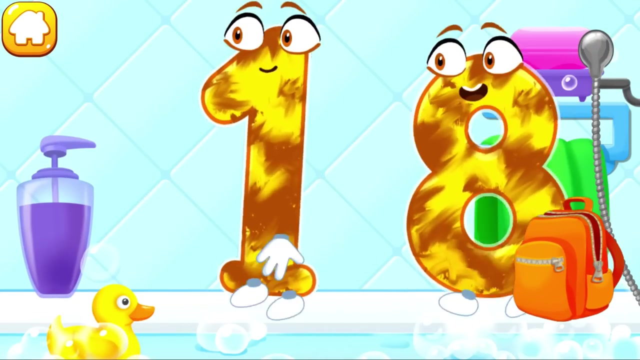 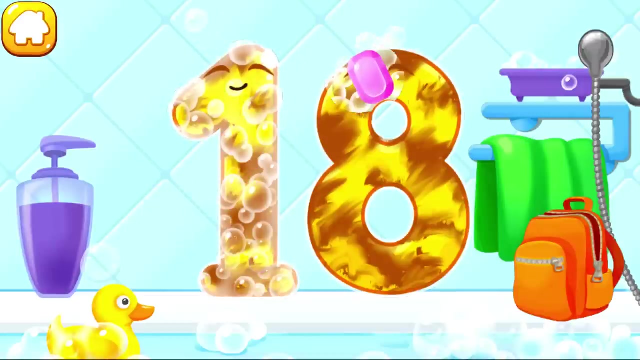 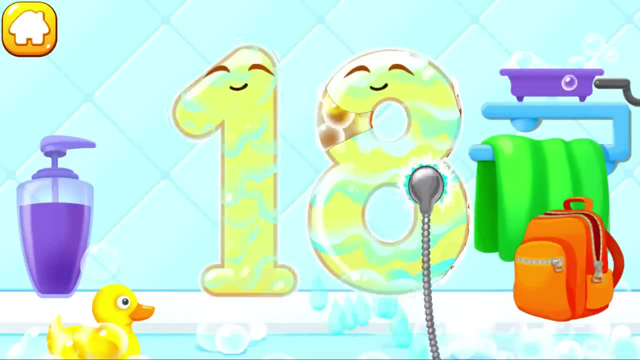 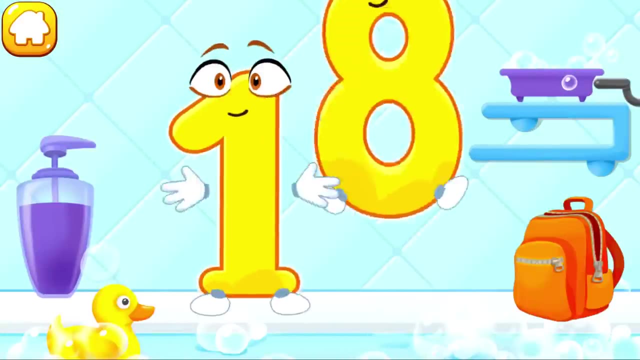 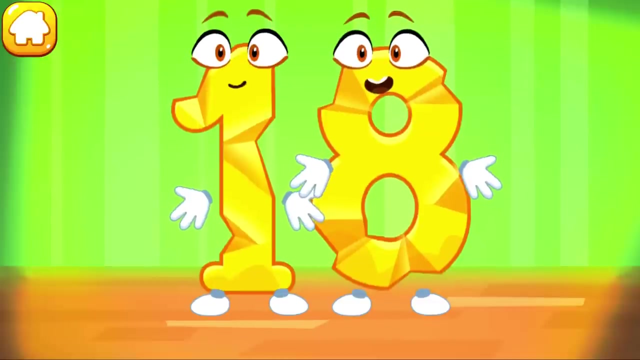 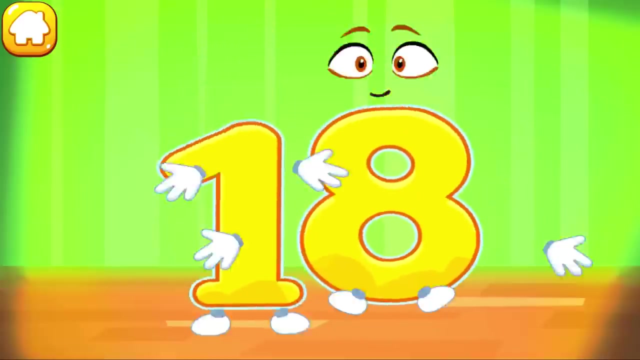 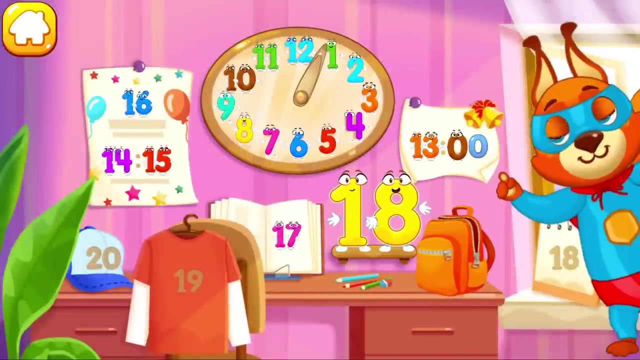 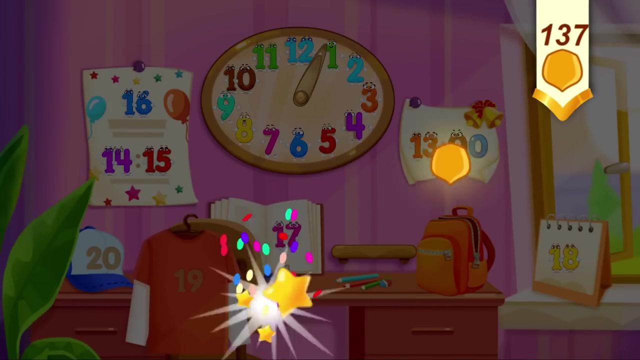 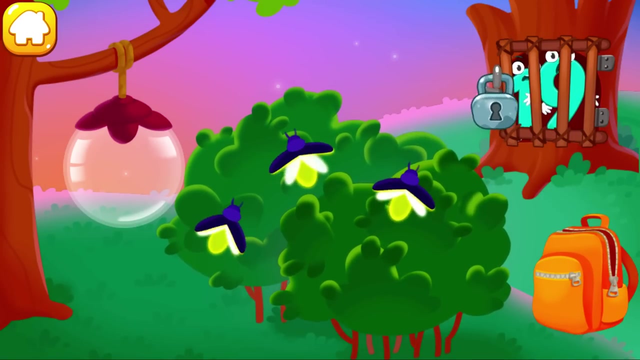 wipe the figure with a towel. cool, smooth out the number 18. good, put the number 18 in its place. thanks, take a nut for the squirrel. number 19 got accidentally trapped at night. we need to light up the lawn to find the key. drag the fireflies into the lantern. 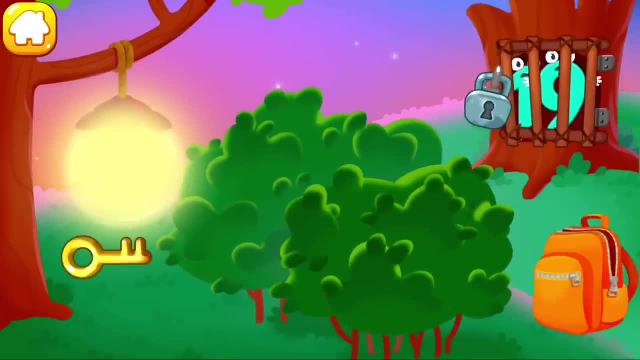 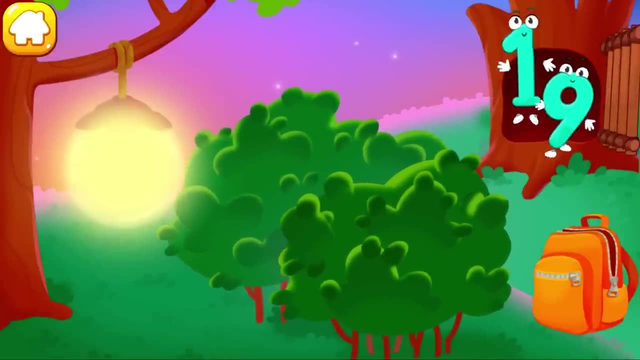 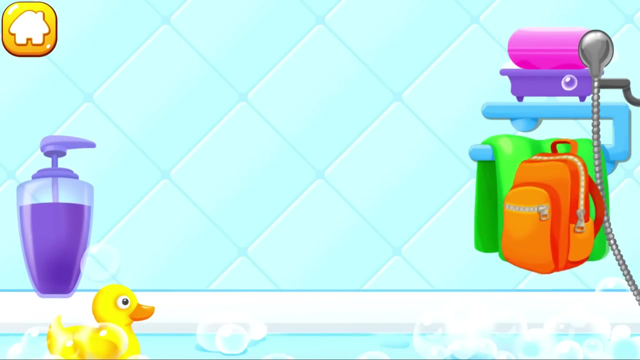 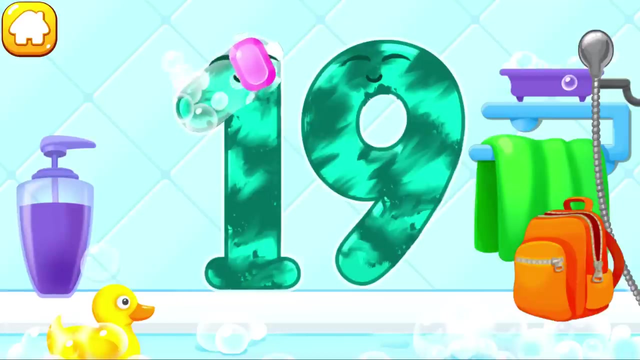 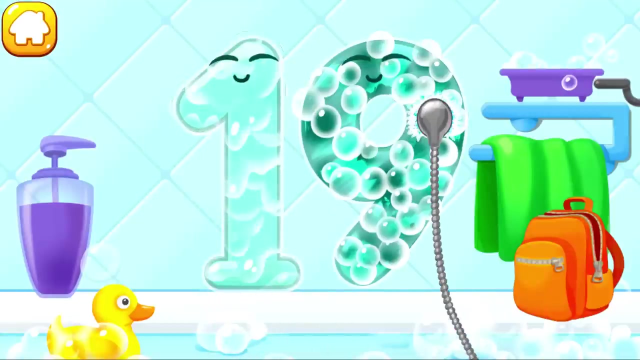 hooray. there's the key. unlock the lock and release number 19. drag the key to the lock and the cage will open like this: wash the number 19 first. apply soap on a number. wash away the soap with water. wipe the figure with a towel. 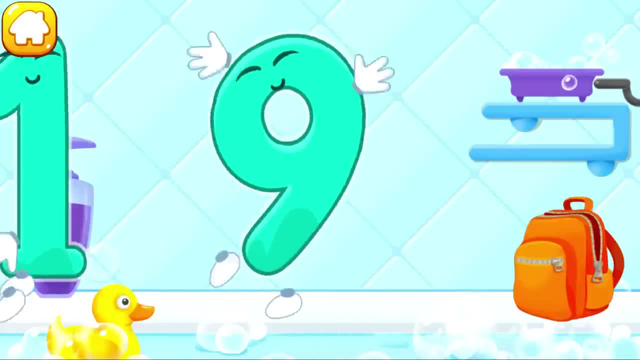 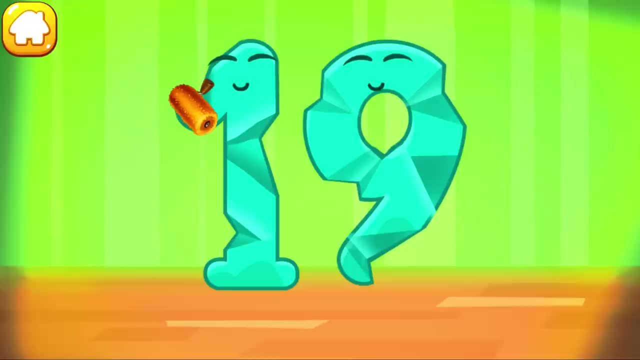 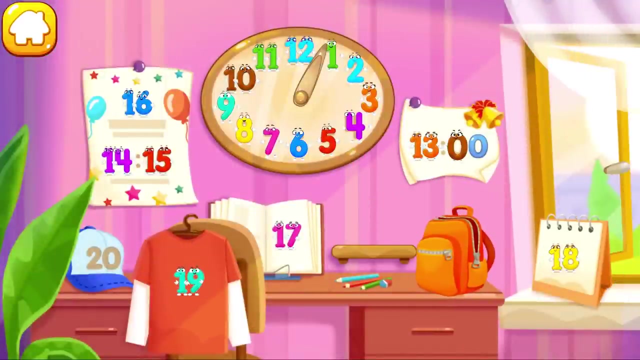 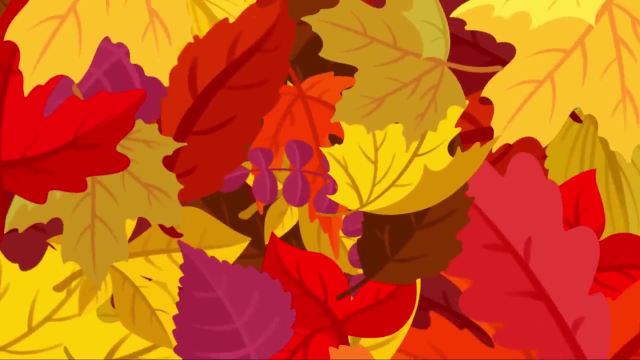 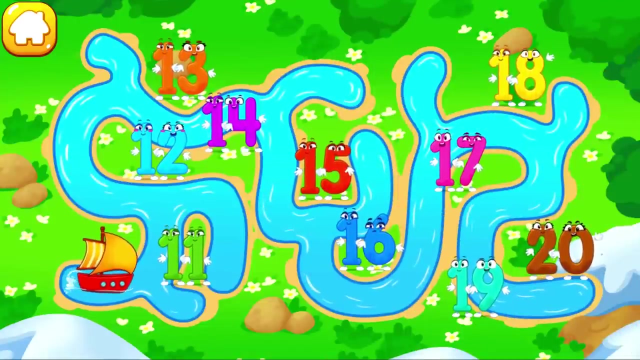 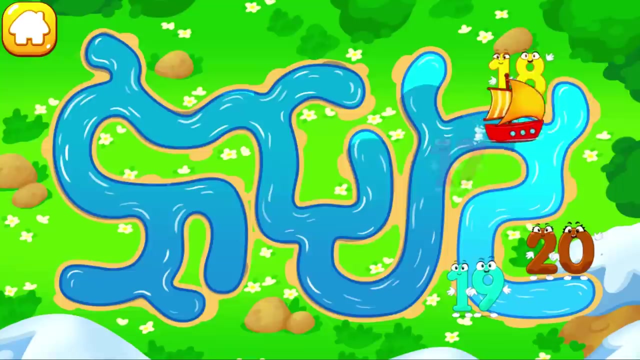 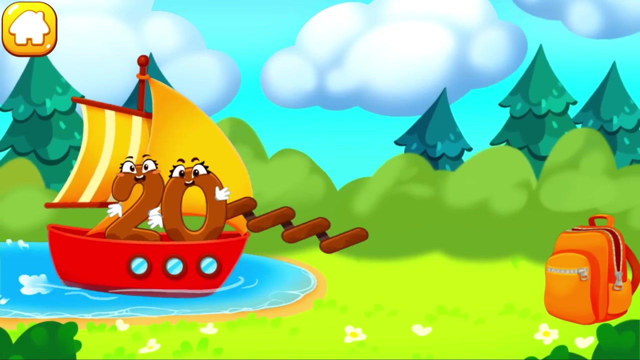 keep it up. smooth out the number 19 giveaway. put the number 19 in its place. thanks for the help. take a nut for the squirrel amazed tree cracker. four. number 20 undertakes a river journey to the backpack. help the boat reach number 20. guide the boat along the river. keep it up, number 20. reach the backpack safe.